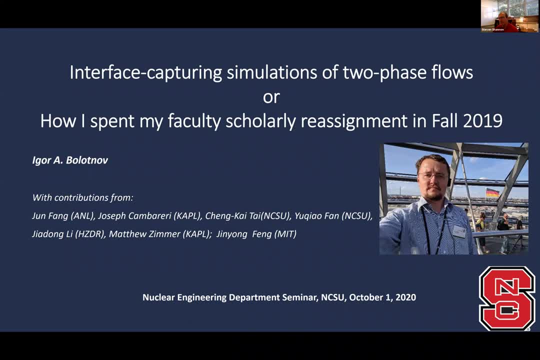 American Nuclear Society and past president of NC State's chapter of Sigma Chi. He has over 120 refereed publications, including over 30 journal papers. He has graduated eight PhDs and 15 master's students through his research program, and it is a great honor to be here today. 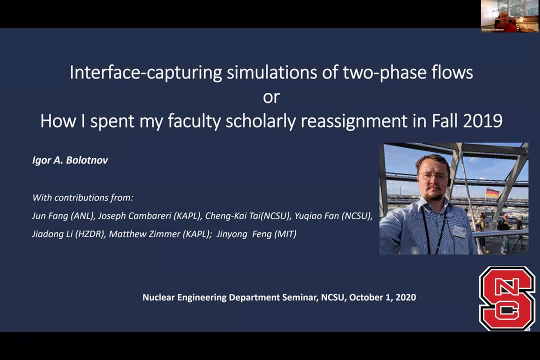 He is currently supervising and advising six graduate students. Let's see. The presentation today centers on some work that Dr Bolotnov did in the fall of 2019, when he was working at HZDR in Dresden, Germany, during a sabbatical that was supported by North 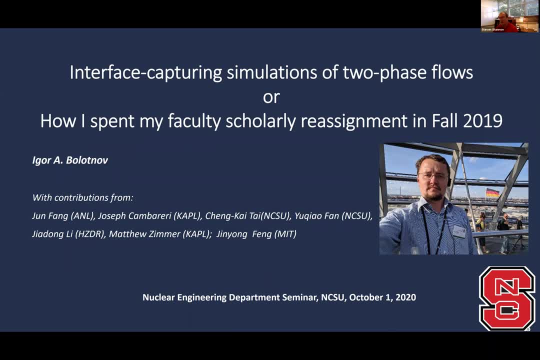 Carolina State University and by the Alexander von Humboldt Fellowship for Experienced Researchers. So at this point I would like to hand the microphone over to our speaker and get the seminar started Again. thank you, everyone for being here. Thank you. Thank you very much, Steve. That's a very good introduction. I don't think I have. 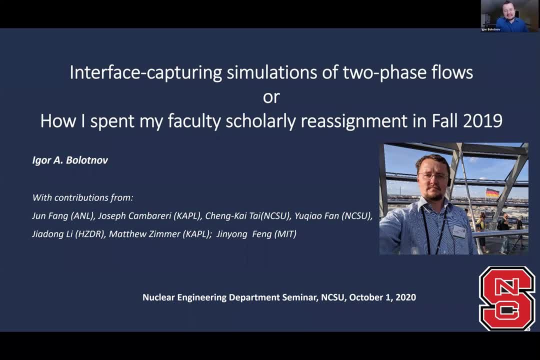 much to add during the presentation, but I will try. So yeah, basically I managed to get a fellowship and I'll talk about a little bit about my experience in Germany, which is a little bit of a little bit of a long story, but I will talk about my experience in Germany, which was very nice. 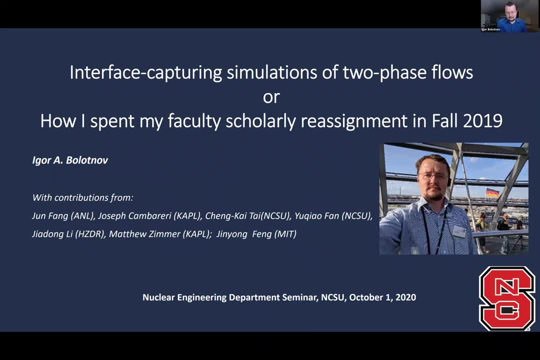 and I'll talk about research as well, and so hopefully this will be a slightly different presentation which we regularly hear, because I will talk about some travel, which now is not very possible, Let's put it this way. So this picture is actually: I'm on top of the German Bundestag. 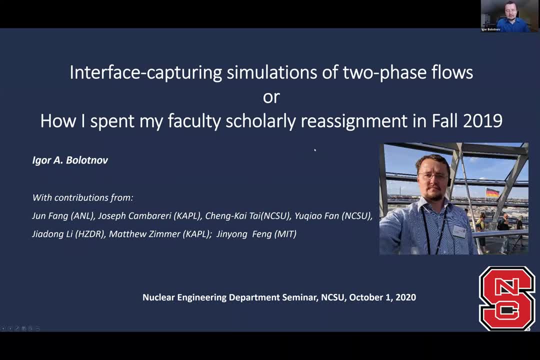 so they have this glass roof and sort of view area. it was when I visited Berlin and actually a couple of times during my Dresden stay, and some of the results I'll show is by my former students, my graduates and current students as well, so at least their name here as well, it's. 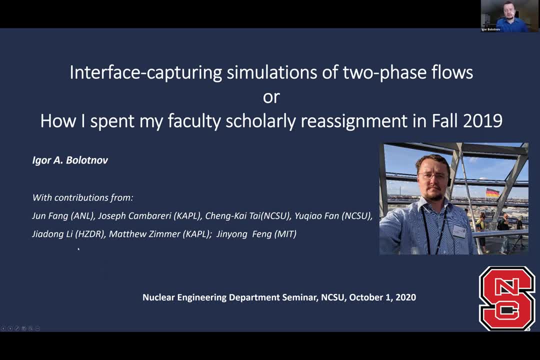 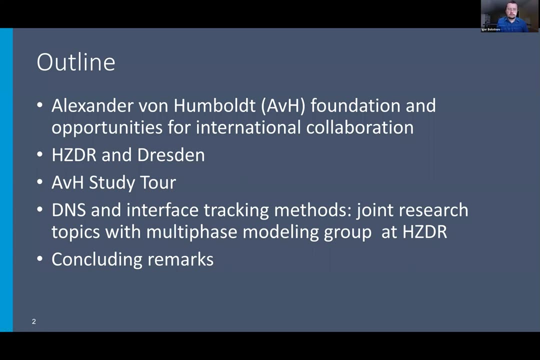 one of the students I will also highlight, who is HDDR student, but we will work together- when I was there- and my throat is a little bit low today, but you know I'll try to speak clearly, okay. so brief outline. I'll talk a little bit what the Alexander von Humboldt Foundation is and and what kind of. 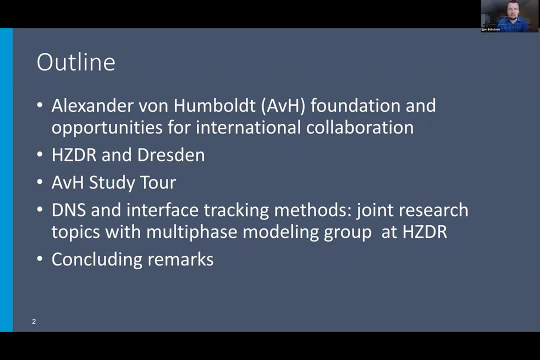 opportunities many of you may have actually from this foundation. and then then how sort of I got into that, and then I'll talk about the HDDR, where I stayed, and there was an interesting thing about travel AVH study tour which I experienced last August. now I'll talk about actual research. 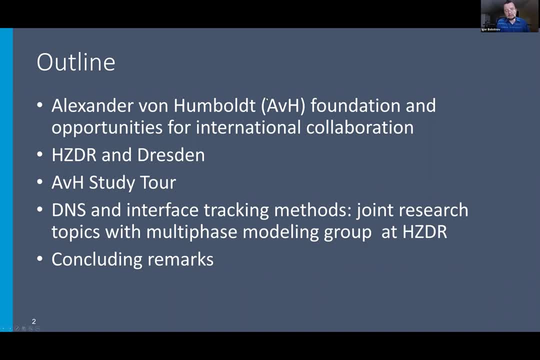 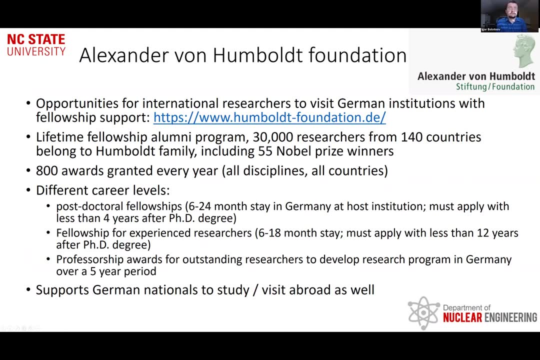 about travel, AVH study tour which I experienced last August. now I'll talk about actual research a little bit, and that will conclude my presentation. so if foundation is a a little bit, and that will conclude my presentation, so if foundation is a German government sponsored entity and and it was founded quite a bit ago, quite 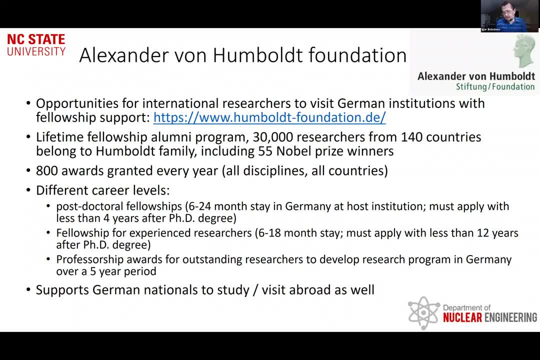 a bit of time ago and Alexander von Humboldt actually had his 250 year anniversary last year, so it was sort of a special year for the foundation and and basically we give out about 800 awards every year year And that is sort of similar to Fulbright, but I think it's somewhat larger scale from. 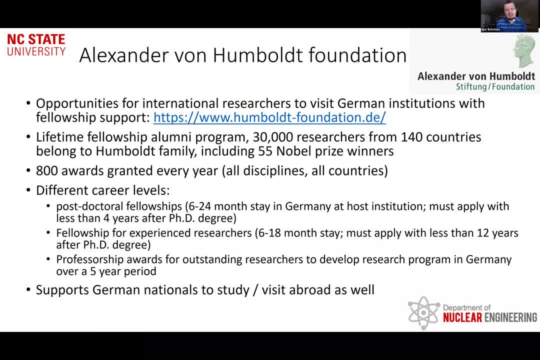 what I understand When essentially, awards are given to researchers outside Germany to come to Germany or it's given to German researchers to go abroad. So basically it's all about the exchange of research ideas And essentially you can obviously read more about the Humboldt. 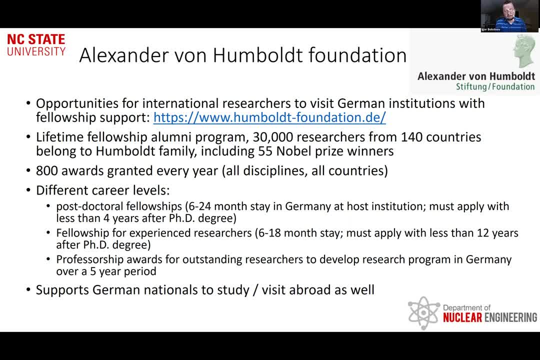 Foundation on the website, But for now we have about 30,000 researchers joining this sort of alumni program which we have And basically what I inquired, that every five years or so I can actually apply for some small grants at least to visit Germany for. 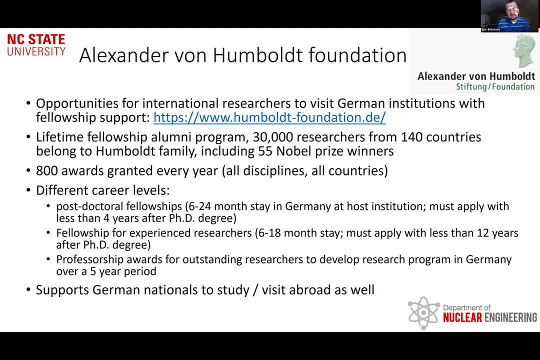 a conference or something like that and they would approve. In addition to what, they allowed me to stay there and paid some stipend. They have 55 Nobel Prize winners. That's very obviously general, so it's not focused on engineering or anything like that. So it's all sorts of area of research which covers the fellowship. 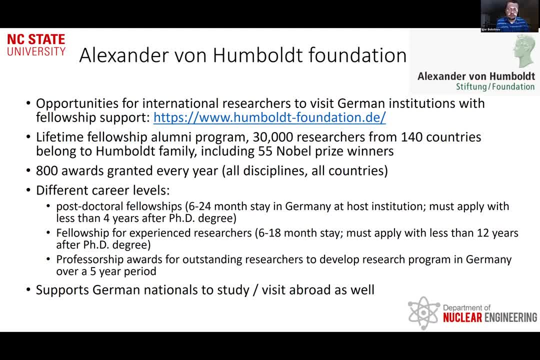 So some examples. So we have postdoctoral fellowship So you could, as a recent graduate- if you're within four years of your PhD degree, you can apply. You have to have a German host, So you have to have somebody who would host you at the application level, right? 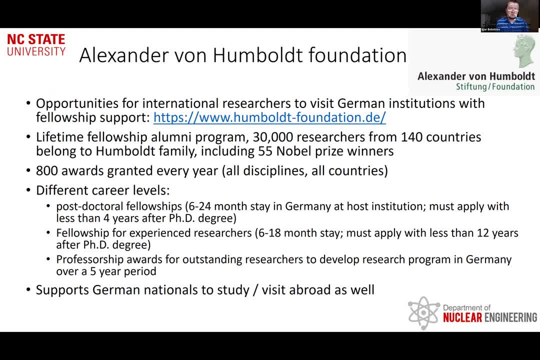 So if you're in my area of research, then obviously I already have some connections there. What I want was this: for experienced researchers, You have to be within 12 years after your PhD degree, And actually last August I am exactly 12 years after my PhD. 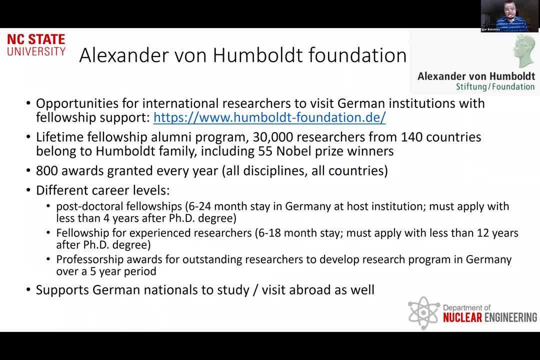 But when I applied I was more like 10 and a half, So it's an application time And there are application deadlines, So you can apply any time you want. once you collect all the paperwork, which wasn't very hard. The proposal was maybe a few pages, So it wasn't plus some. 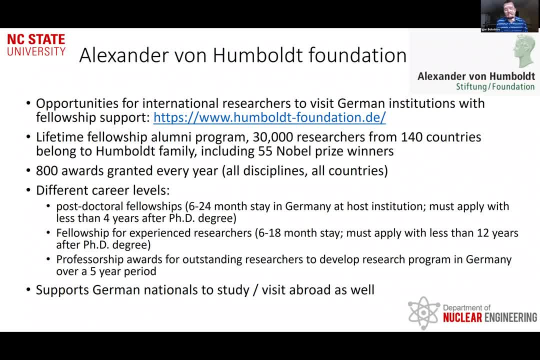 some other information. So I mean the technical part of the proposal, what we want to do- And there are some very, very prestigious awards for senior researchers when they can issue a professorship- And basically it would be some substantial funding. 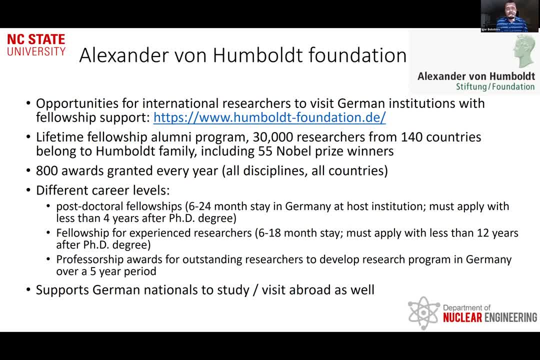 So it would be around four to 5 million euros, which is sort of the same amount of dollars. But you know, if you're selected for that you would. you would basically have to go there for five years and really develop the lab, And so that's- that's not just your salary. 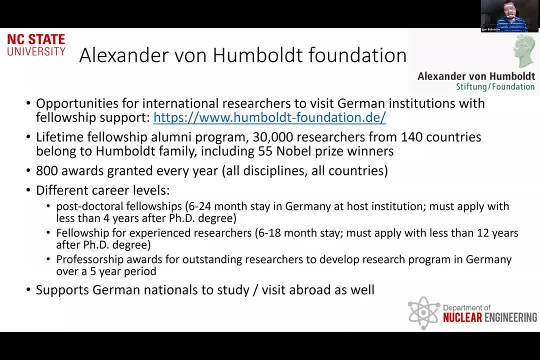 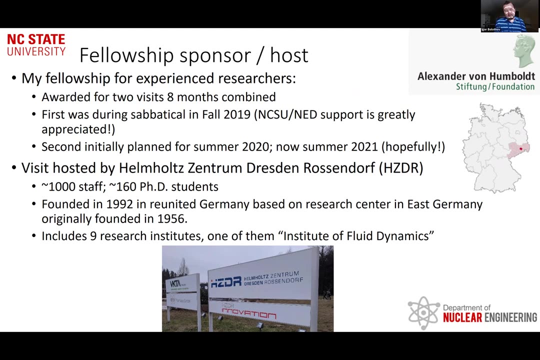 obviously this amount, but it's basically very, very nice startup. Let's put it this way. So this is, this is for for very accomplished researchers And, as I mentioned before, it's it's really the exchange of individuals. So specifically what? what what I got is is: 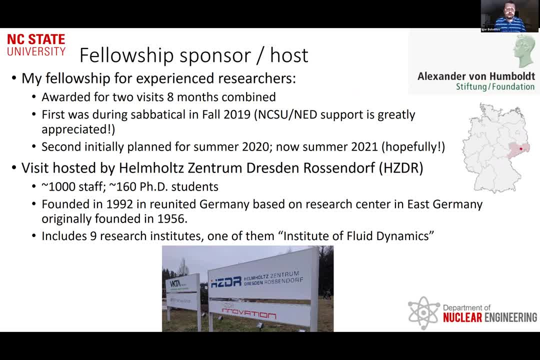 fellowship for eight months combined visit and the plan was to go on sabbatical for one semester. So I appreciate the support of the nuclear engineering department and state. so so every faculty typically eligible once in seven years or so I think, to take sabbatical. 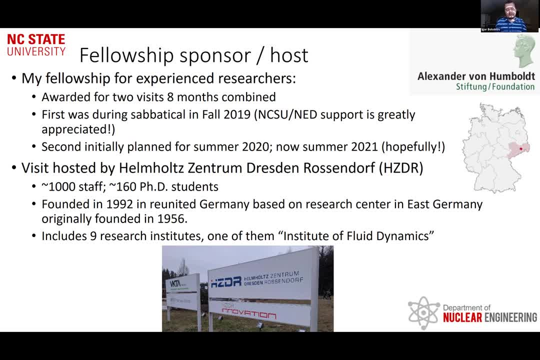 Not everyone Takes one. So you know I encourage faculty to consider those opportunities, especially in our department, as we're grown now. So this should be somebody to teach your classes if necessary. But obviously you know department head is a point of contact for that. And then 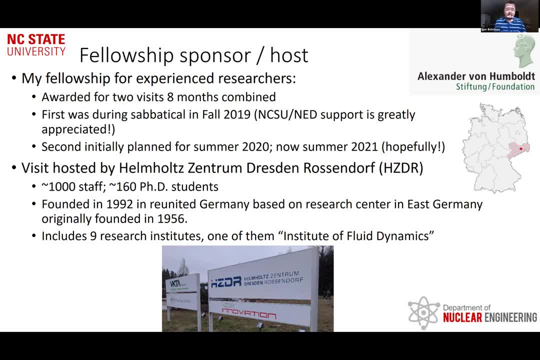 I plan to stay in our three months during summer, in summer 2020.. That got postponed. Now I'm not 100% sure 2021 will happen, but we will see, I guess. So, um, now you know. 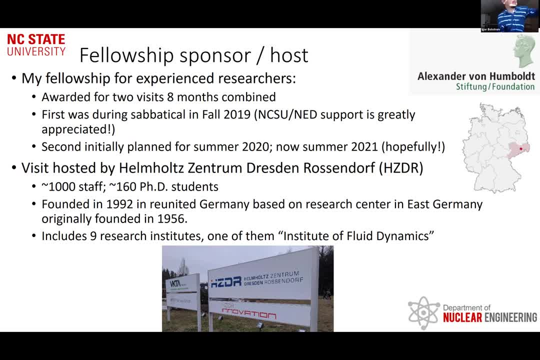 I went to be a second, Just this little bit. I went to the Helmholtz Center on Dresden-Rossendorf, which is in East Germany near Dresden-Rossendorf is a village of two houses basically, but historically that was sort of a research nuclear reactor site actually, when it was founded in the old 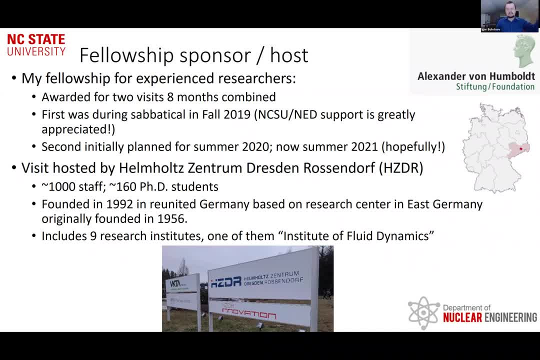 days in 1956. And so we positioned it about, you know, 15 months. And then it was repurposed. So we went to Germany and in the beginning of the year and it was repurposed And we ended up in Germany And we recently went to Germany and then in the beginning of the 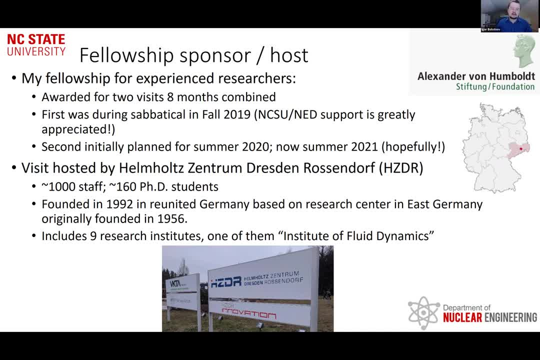 from CC Center and in this sense are kind of similar to our national labs, which are typically in the middle of nowhere. it's pretty big, the thousand staff, about 160 PhD students with those research centers cannot grant PhD degrees. they typically collaborate with universities. so TU Dresden is sort of. 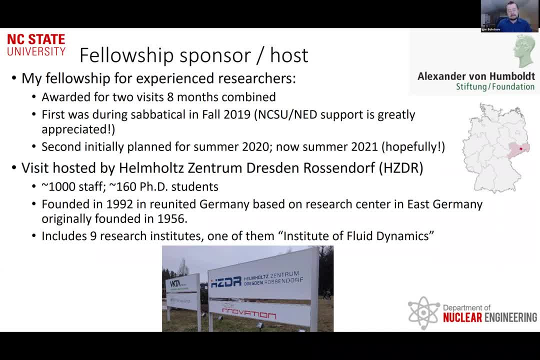 typically to go University and essentially be students spending a lot of time at the research center. again, like some, our graduate students are spending a lot of time at national labs and in HDR there are nine research Institute's, but but you can imagine if it's nine out of thousand staff. so is a. 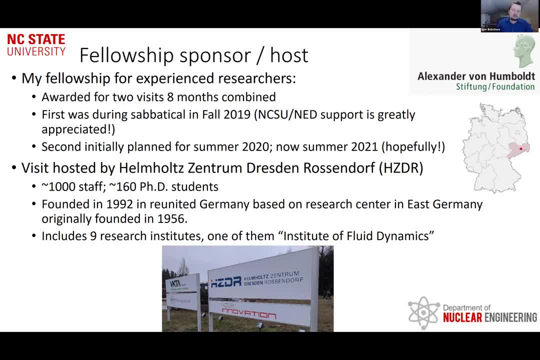 hundred staff in each Institute, more or less one of them Institute of fluid dynamics, and then the group which I was working was more like 20 people, including students, 25, and that's a computational fluid dynamics group which was, which is headed by dr Lucas dirk Lucas. 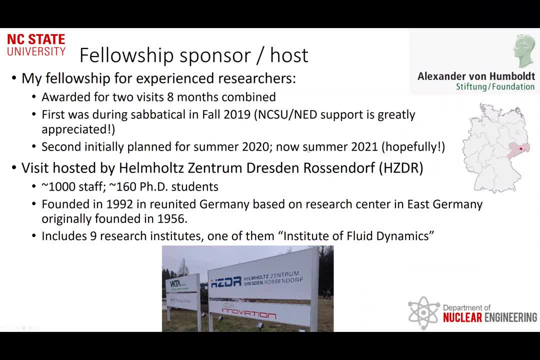 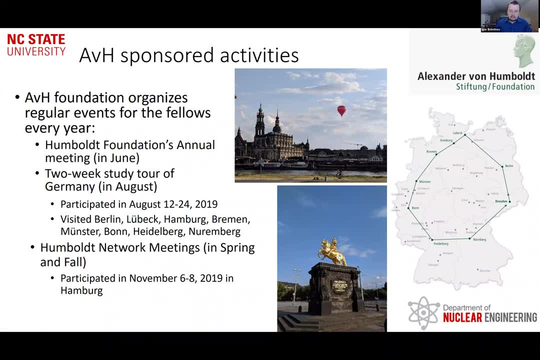 this. you know, I'm not sure if I can say that. I'm not sure if I can say that. I'm not sure this was my host. so one of the interesting things I want to talk about before going into research details. so so, if you are selected to for this award, 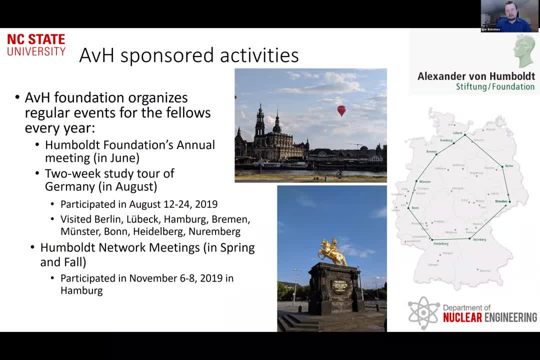 there are a few interesting opportunities to get to know Germany a little bit better, and and and. so under the new conflict of interest rules at NC State, this is considered- what is it? foreign government talent recruitment program. so now I have to fill up those forms because, well, you know, foreign government gave me a little bit of money. 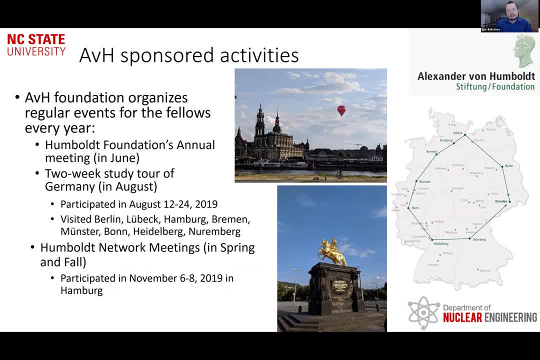 to learn a little bit about foreign country, right? so, and basically, one of the things which we do is is an all meeting of the Humboldt Foundation, when we have a so-called study tour of Germany- and I'll talk a little bit more about that, what, what I participated in- and they have network meetings and they 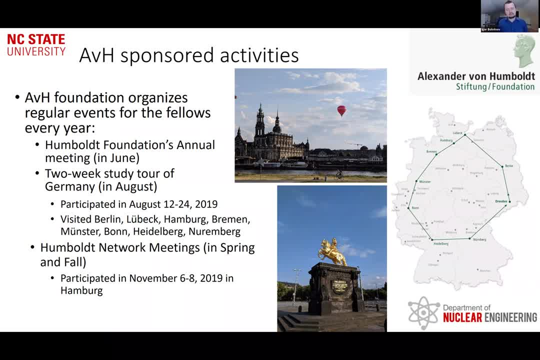 get together or they have a meeting with the German government and they have a all the fellows in sort of the same location- this time it was in Hamburg way- where you basically interact and learn a little bit more about each other's research background etc. so it's kind of interesting experience because, again, you 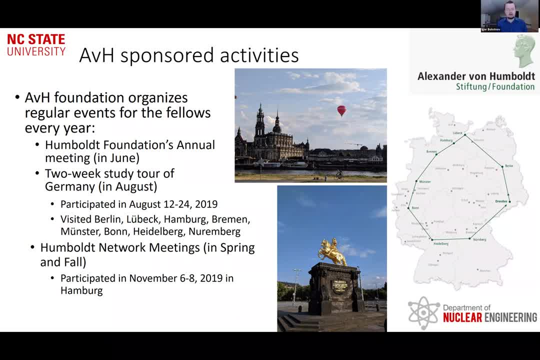 have those fellows coming from all over the world. so, for example, the year I was awarded this fellowship, only five researchers from us who awarded the same level of fellowships, and then more postdoc researchers. so but then they. this, you know, basically, in many different countries people come home, and so this: 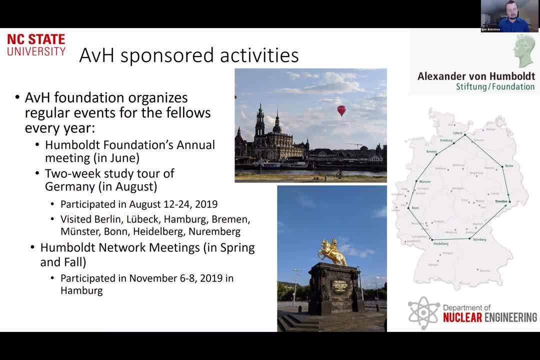 two-week study tour. I will, I will. I will give a little bit more details what I saw in, but on the right you can see the map of Germany. and so we took a bus basically, and we spent two weeks on this bus, but not necessarily on the bus. but 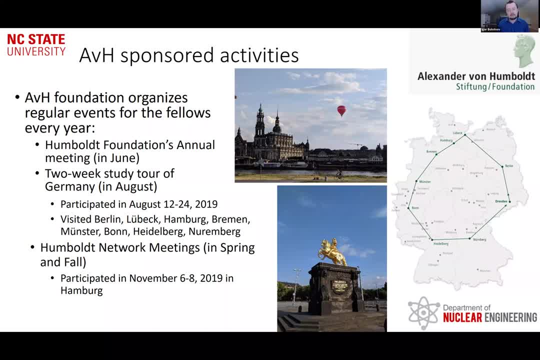 you know two, three hour rides between the cities and then a lot of the other countries of tours. that was very enjoyable but actually hard work. so they didn't allow the kids to come. they would only allow the significant power to come, but because my wife had to stay with. 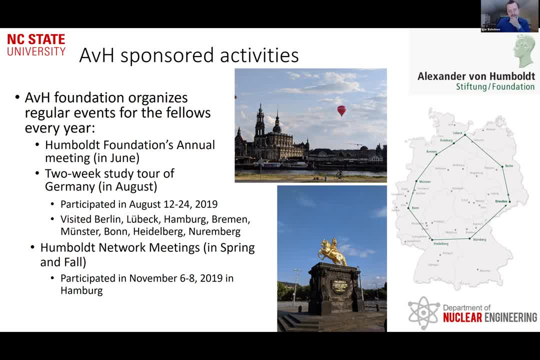 the kids. so actually i i traveled alone. um, interestingly enough, uh, just how it tells you that the world is pretty small. um, i've met another american professor on that bus and we kind of, uh, uh, communicated quite a bit and and he was, uh, from a building across, uh, the uh. 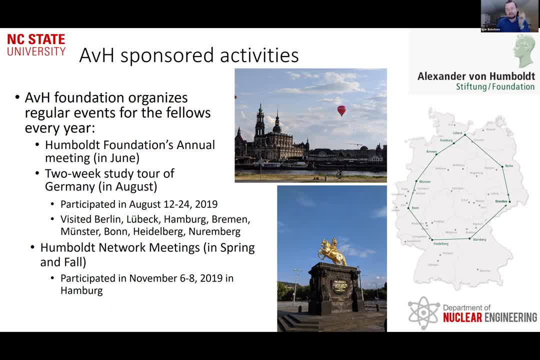 from engineering building one, basically, so from nc state. so, out of all the people, 20 people who were interested in the bus. so so joe tracy is a. he's a professor of, i think, materials at nc state. um, we will know our american professors on the bus. so that was interesting. 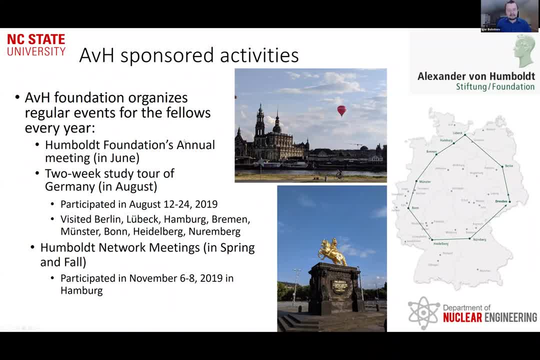 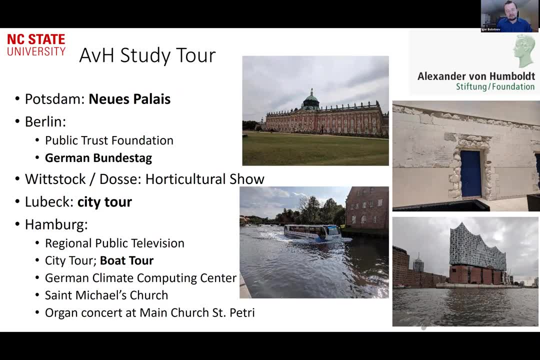 so nc state you know kind of was well, well represented, um and uh, um. just just a few pictures, uh, uh. so we travel to potsdam. so this is sort of a very historical place in germany, uh, with palaces and again, compared to us, a lot of history. that's kind of impressive, a lot in in berlin i you saw a. 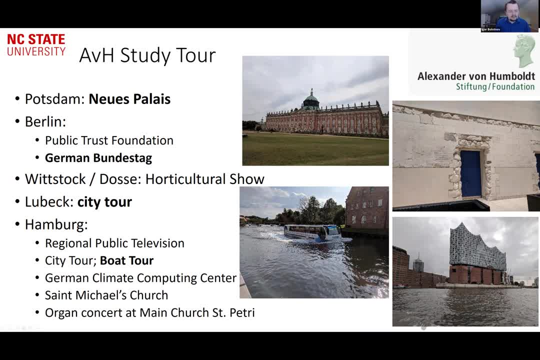 picture of german bundestag. so this, this is, it seems, like a- i don't know how well you can see, but but but the top uh, top uh right picture. so this is the door uh of the um german chancellor's uh uh office when she uh. 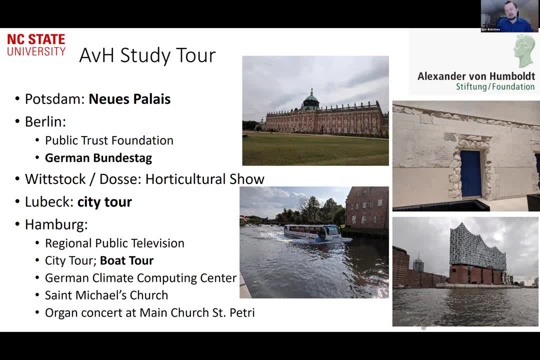 angela merkel goes to bundestag um, and this is a historic building and part of history was the world war ii, so so the writings on the wall actually by russian soldiers from 1945, so it amazed me that they preserved history and you know um so that that's interesting. so when there 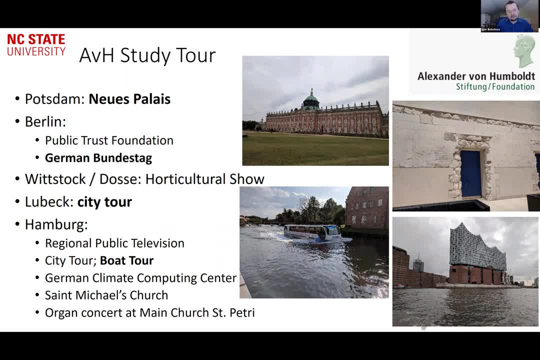 are some other city, uh, cities like lubeck, uh, we, we're going to talk about that in a little bit, but we, we, so we got some city tour and it's actually i went for the program just to show some things. hamburg is we spent spent a couple of days there. on the bottom right picture you can see the 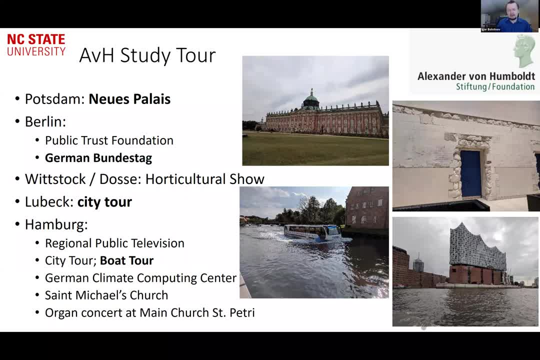 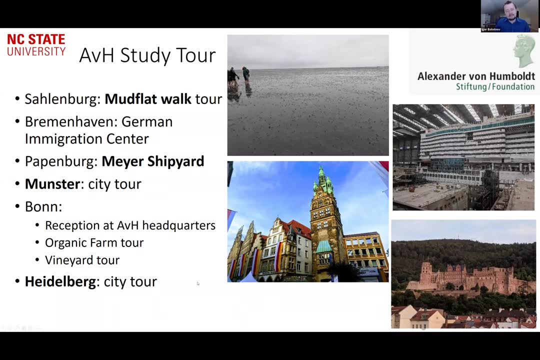 hamburg: uh, opera house. that's like one billion dollar project to to uh, quite, quite an impressive architecture, but this is uh sort of a mix of modern and um historical germany. um, there is an amazing place on the northern germany, in salingburg, so we had this smart plot walk tour. so basically you have the. 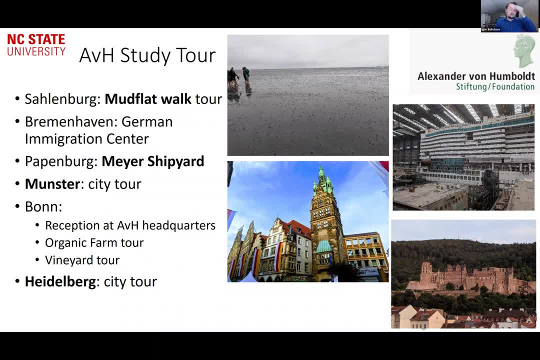 ocean, uh, um, which, which really you know two days ago, twice a day, right the, the shoreline goes away by by 15 miles. so you really have this, uh, you know a few feet of water during one part of the day and then you know 15 miles of of of this month for the other half a day. 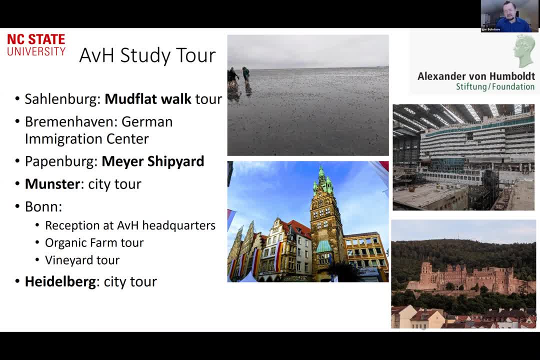 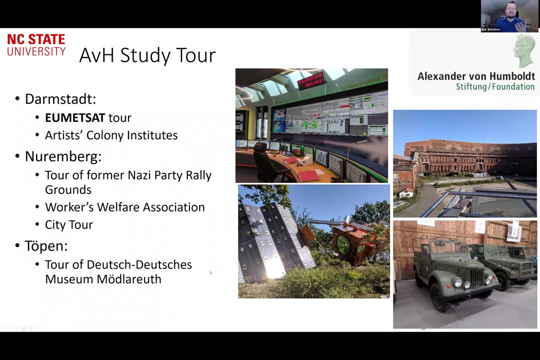 um, so so, visit the mayor shipyard, so, so, um, construction of one of the largest uh cruises cruise ships. so that's a picture on the top right. um, heidelberg was a awesome city. um, so that was, uh, one of the older castles there. so now, you know, and this tour was kind of very, very diverse, so that's what. 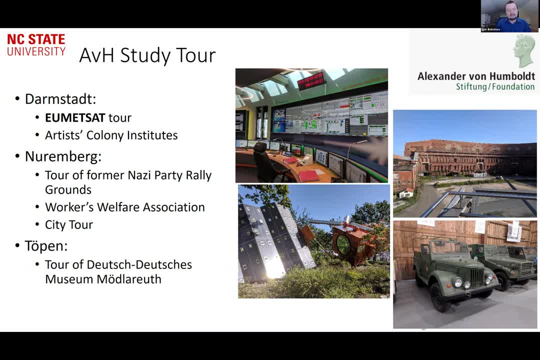 i'm spending a little bit of time on that because it was it's something i would remember forever, i guess, um, uh. so so we we visited, uh, uh, the um meteor station, which which controls the meteor satellites, and it's basically um, gets the weather information for, for, uh, european union, uh. we visited nuremberg, uh, so they had uh. 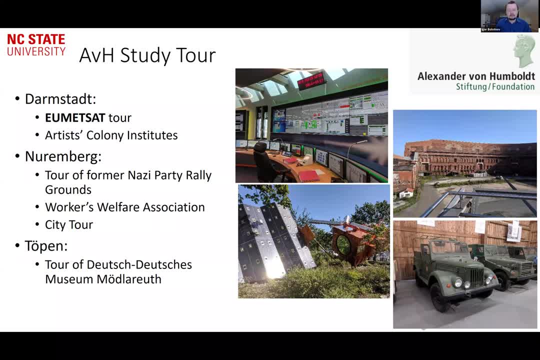 some, some again historical um buildings. so this huge coliseum which um nazi germany uh was building but didn't finish uh and basically it was for for the party rally uh grounds. so very, very impressive in terms of the size and um, and they're also in some, some other places. 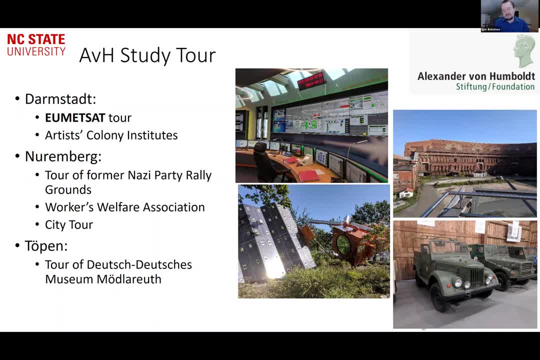 so, on the bottom bottom, uh right, so, there is a village which was separated, like berlin was, but but by the actual boundary between eastern and, uh uh, western germany. uh, during before, before before you, uh wall fell, And so we had, we had the, the alternating military vehicles from: 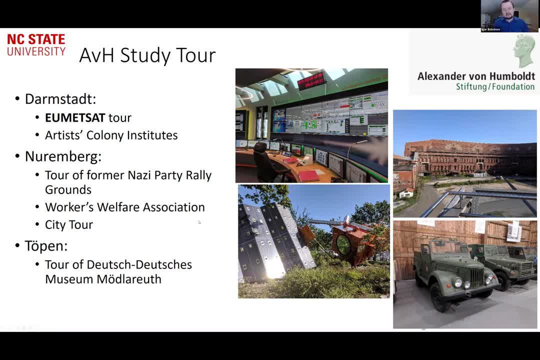 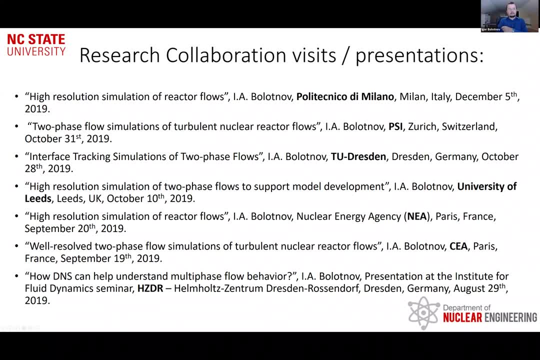 from Russia and Western ones as well. So it was, you know, I think, All right. So, besides, besides that tour, what I also did- and I also actually I got some support for three of those trips from College of Engineering Faculty- 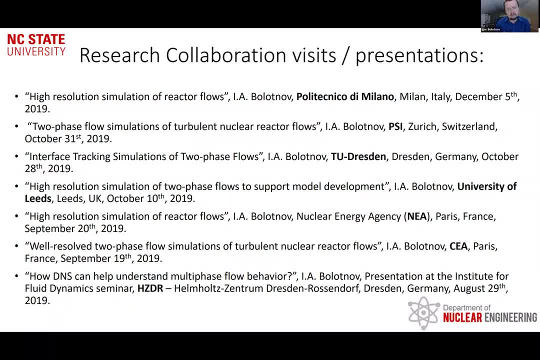 Faculty Advancement Office headed by by Christine Grant. So so I kind of once I got the fellowship, I did some planning And so I visited and gave presentation and kind of develop additional collaboration. So going from so, this is actually reversed order. 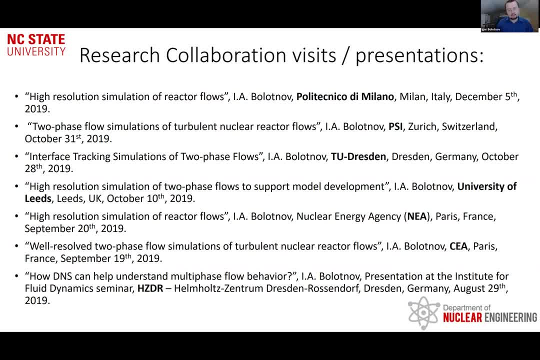 how I put it in my CV, but so, so, obviously at HZDR. so I made a presentation about what I do when we visited Paris and I visited CA and NEA with in two days essentially, And then actually flew to England University of Leeds. 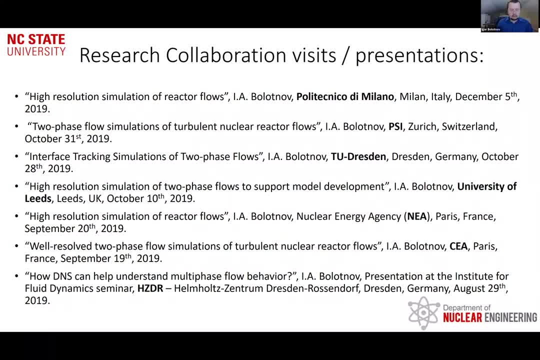 which is a strong group doing multi-phase modeling and simulation, And actually we have ongoing collaboration with Dr Marco Colombo. there. He has his own fellowship and I don't know if anybody attended, but I think he was the one who presented the last in-person seminar in our department. 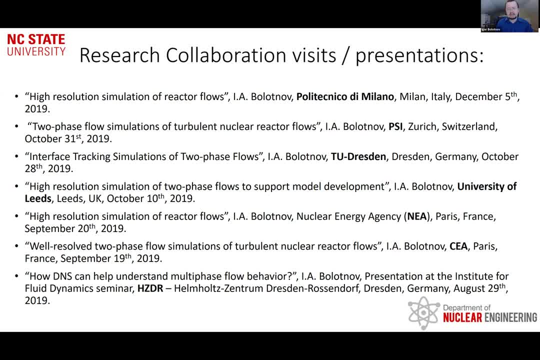 on March 12th or 15th or something like that, before, before COVID restrictions. So so he he had the chance actually to visit in the last moment. So TU Dresden is this sort of a university which we collaborate with at HZDR. 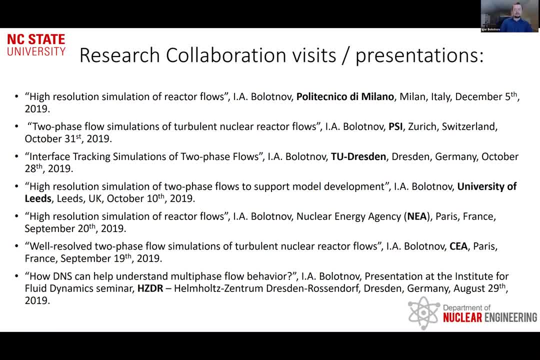 in terms of educating students and grad PhD degrees. I visited the PSI and ATH Zurich later on to have some good discussions. I'll have small slides on that. And finally, I had a chance to visit the Milano. We had a couple of meetings. 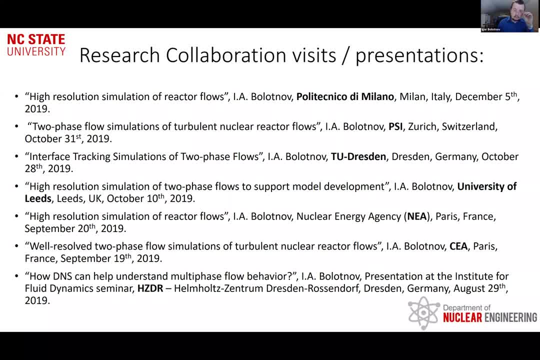 also quite, quite strong um, a nuclear relevant research done in in italy and everything is so close in, uh, in europe, obviously it's different states is like different states here, right going to georgia here, it's like going to italy over there, um. so this is the same list with some some. 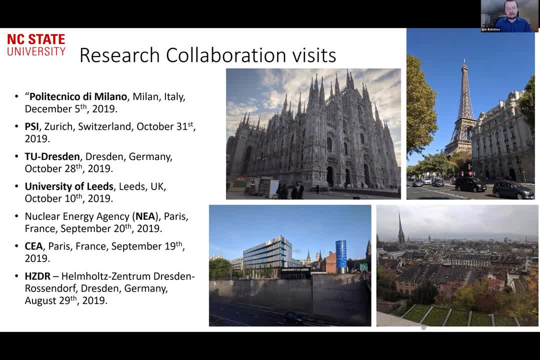 pictures: uh, uh, to proof, i was actually there. um, university of leeds is actually. the area is somewhat similar, i think, to, to rdu research, triangle park and whatnot. in a sense it's sort of uh away from major historical centers, but but because of that it's growing uh. 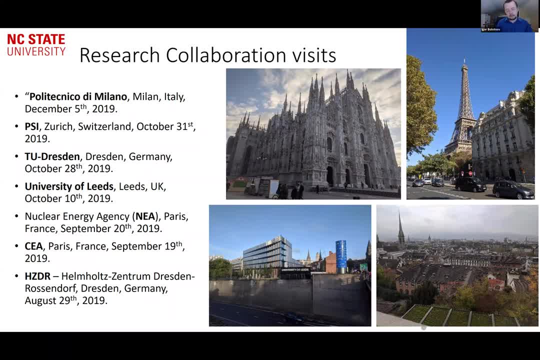 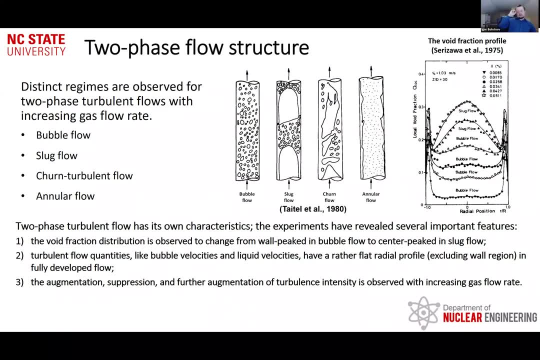 technologically, and then you from educational perspective, very well, um, all right. so now what i when i want to do. i want to briefly kind of talk a little bit details about my research and then i'll i'll present some of the projects which were started during my collaboration. there were some quite a 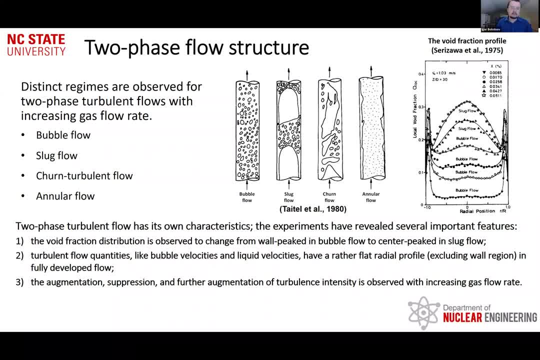 few different ideas developed, but obviously you know, when there are no results, publishable results yet, i i'm not going to talk too much about those. so two-phase flows, um, um, essentially very important for uh, uh, for for reactor technology, for for boiling, but also for chemical engineering and 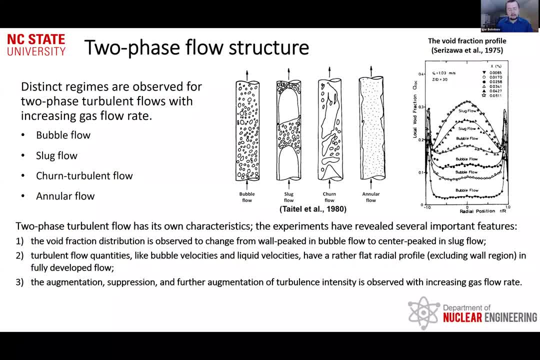 other things. so one, one of the things which i didn't mention in terms of this fellowship: germany, as you may know, is not very, not very kind to nuclear energy, so they don't want it. so, so and so to get this fellowship, i applied in the fluid dynamics, basically area, but nevertheless, hddr is actually historically 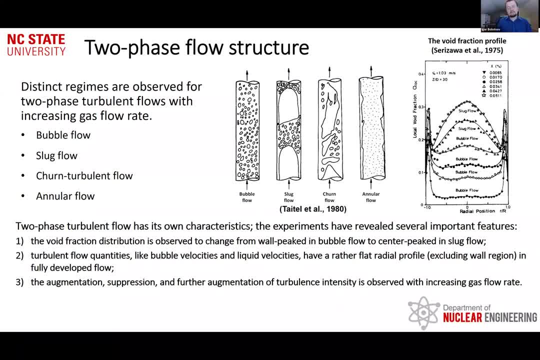 again nuclear engineering institute, so we have nuclear safety divisions, they have computational fluid dynamics, so it was a very nice experience in that sense. um and so. so we challenge with flows of bubbles is: is they they really um, behave differently in different conditions? uh, temperatures, pressures, uh, concentration of bubbles and um, uh, what, what? what happens essentially is: 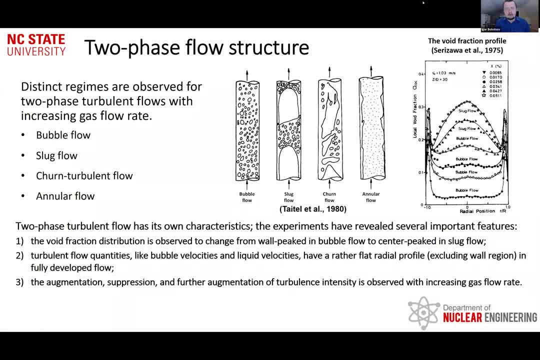 that, um, i'm okay, sorry. i just saw the chat window popping up um and and and so, um, to be able to predict the behavior of the flows uh, different modeling approaches uh can be used, and and the balance between the modeling approaches. you either have uh low resolution and have to put 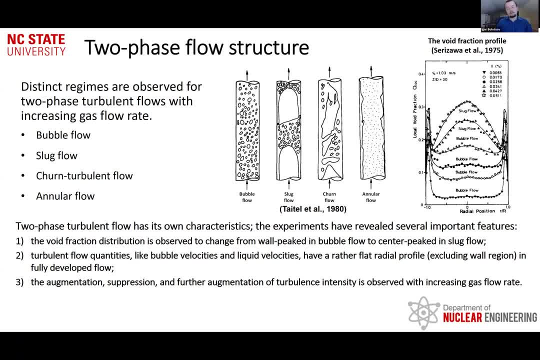 a lot of either empiricism or a lot of high quality models into in order to have a good predictive capability of um a lot of important phenomena such as departure from nuclear boiling and nuclear safety, um, or you can kind of use extremely high resolution simulations in order to 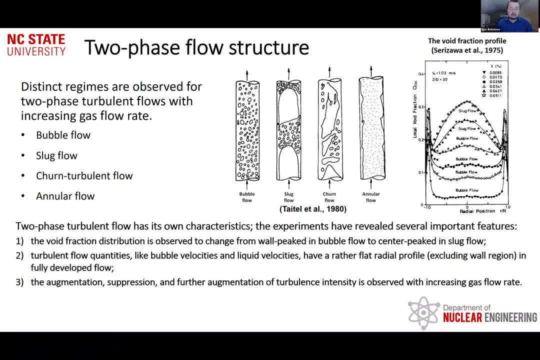 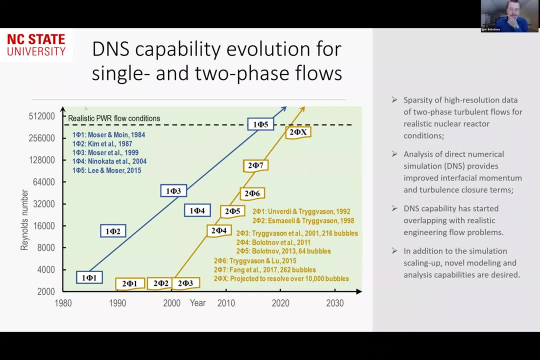 resolve all the features of the flow, including the interfaces, um, and then it allows you to have universal predictive capability. but that comes at a huge and often unaffordable computational cost. in my group, what we are benefiting from is the fact that you know, computational resources become more and more um affordable and this way you can actually utilize. 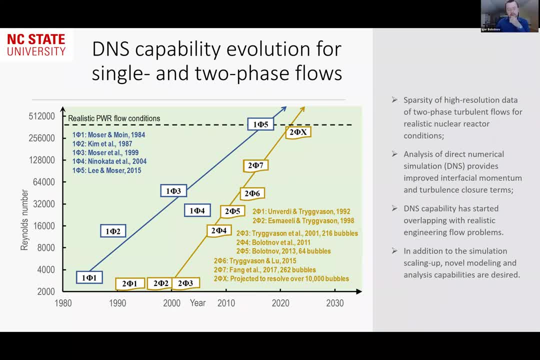 the so-called direct numerical simulation approach, when you resolve all those features and essentially can perform virtual experiments, uh, in order to study different phenomena. so in this plot we are looking at the reynolds number, which is, you know how much turbulence you have in the flow versus um single phase and two-phase type of capabilities and and 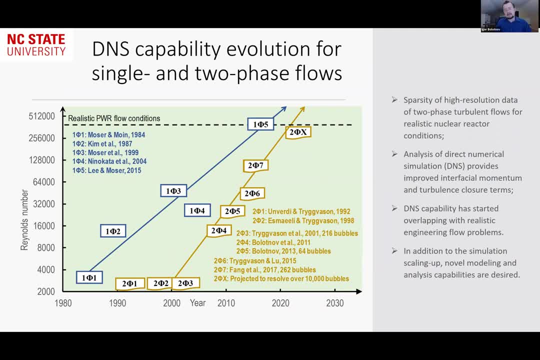 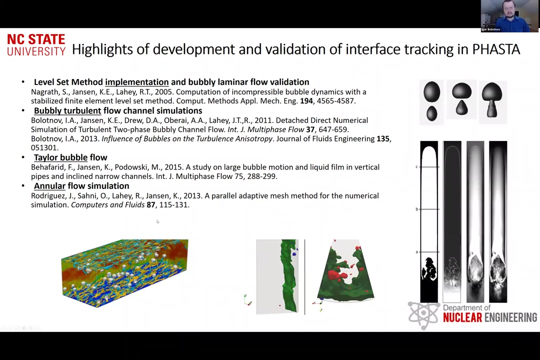 and what was done over the years and and technically we we are now sort of on this border where i can do, for example, realistic pressure reaction and so on. that data is not so much about the amount but just like how cut off the flight time. it's basically no difference on when the temperature going down and down and so on and so forth. so we can also use this, and we will just use these examples here, to demonstrate what the reactor conditions for uh for for many flows, however, it's still, uh, a sort of a table top type of experiment, right? so the domain size is nowhere near uh, the reactor size, right? so you would look at single sub channel, maybe a few of those. 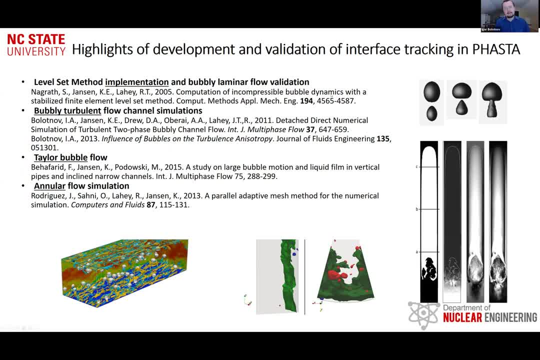 student. I didn't participate in this project, I was doing something else back then. but the level set method, which is one of interface capturing techniques which allows you to track the liquid gas interfaces, was implemented in the code which we still use. but later on, as a postdoc, I did some first-of-a-kind 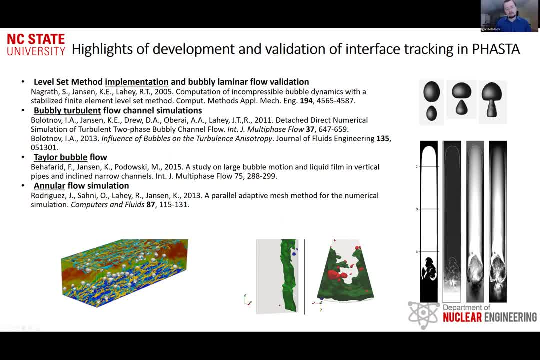 public flow type of simulations to study the turbulence influence on the on the flow. and then we there were some additional projects- I was not part of these two- when the annular flow and the Taylor bubble flow was simulations were performed, which is again related to to the bubble flow simulations. and then 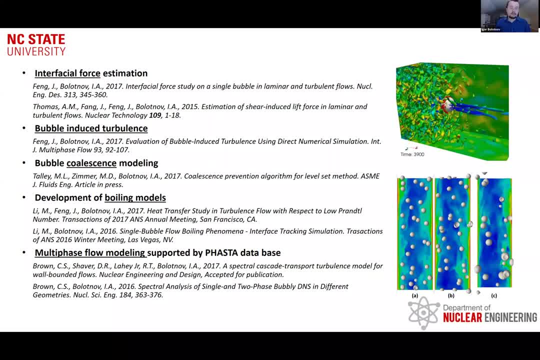 later on, we did some, some. we got some different finding from different agencies, and so we looked into bubble turbulence interaction. we looked into additional analysis of the bubbly flow and many other conditions considerations such as boiling coalescence, contact angle. so so there is a lot of physics which you need make sure that you're representing correctly. 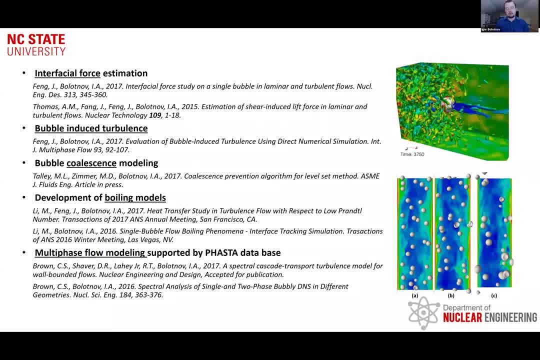 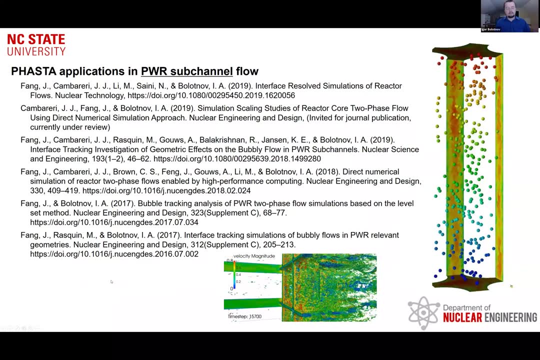 if it's beyond your scale, such as contact angle, you have to produce appropriate models which will be able to mimic this physics, but then you have to verify and validate those models and, as part of a castle which for- and I think that we just síma- is working, and so i would like to remind 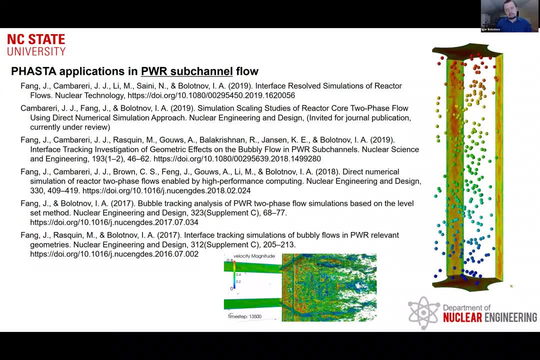 everybody and to say it's excellent. since we started off the tutorial, read that and also it's something that we learned, especially sinceresearch study published back these recent this year- that you can go online, you can download Googleistry, you can go to肉 group and get some 28 S. 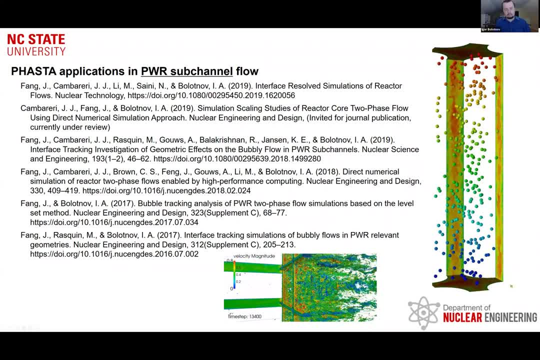 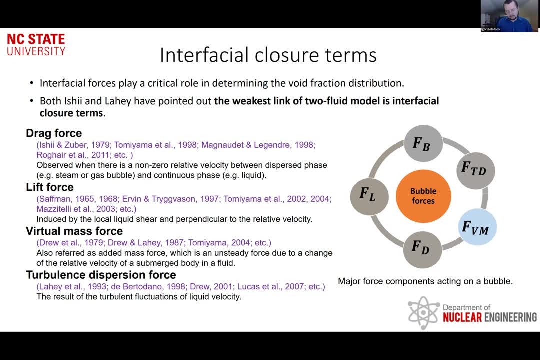 these simulations are expensive, So we published a few papers on that. So one of the examples I wanna focus on and that's what kind of important in multi-phase modeling. So if you wanna go to a larger system which is more applicable to actual applications, 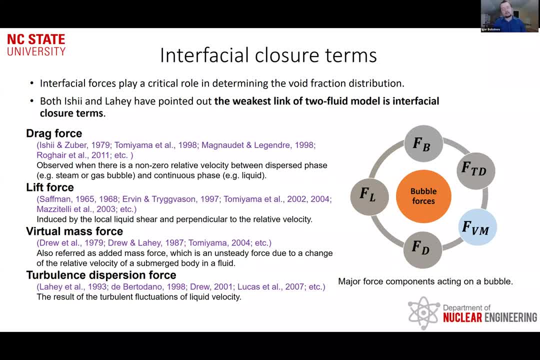 again, it's very hard to use a full resolution direct numerical simulation. You have to typically use either multi-phase CFD or even a coarser type of approaches such as sub-channel or system level modeling. If you look at the bubble, which you can resolve at a very large expense, 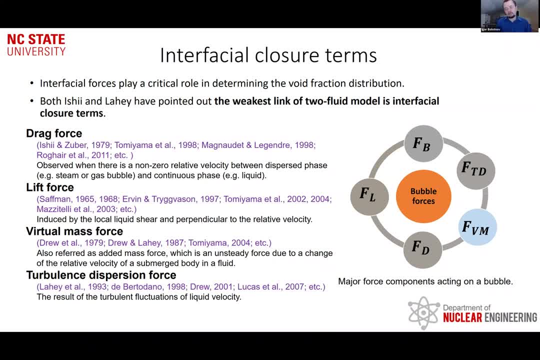 or you can assume some sort of concentration of bubbles. If you assume concentration of bubbles, which is sort of a smooth probability function, if you know what's the probability of bubble being there, then what is very important is so-called closure models or interfacial forces. 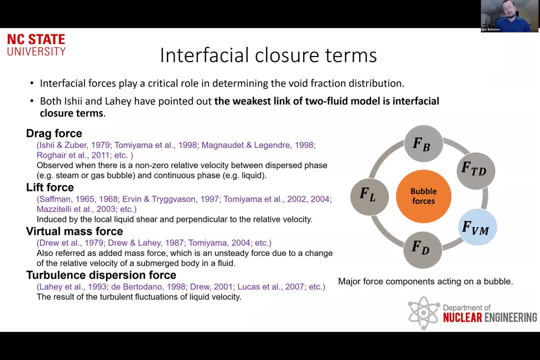 And so I'm don't have enough time to go into too much detail, but the basic idea that there are several interfacial forces which are acting on the bubble when it's traveling through the liquid or in the bubbly flow, and having good models will allow one. 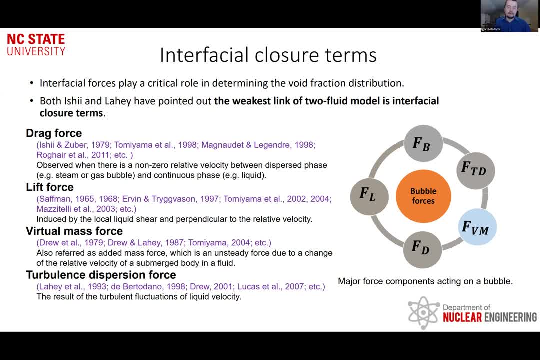 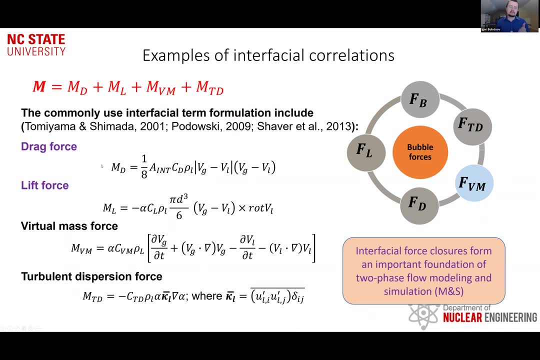 to properly reproduce the two-phase flow behavior in a scenario when you do not actually resolve the bubbles. So, and one of the classic type of models again, just an example. for example, a drag force, it's the same track as your particle. 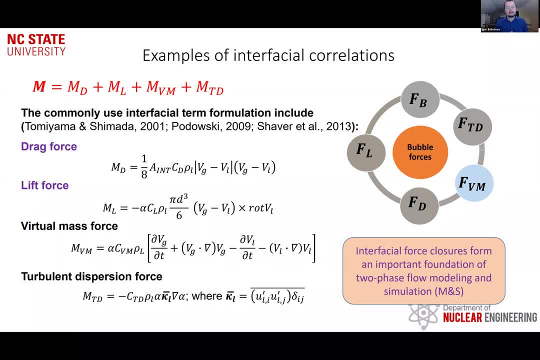 will feel in the flow or airplane will feel in the flow Depends on relatively velocity, squared, but something like drag. but something like drag, firefight is an important component. Leave force is another component than there are other forces, and these are the typical closure laws. 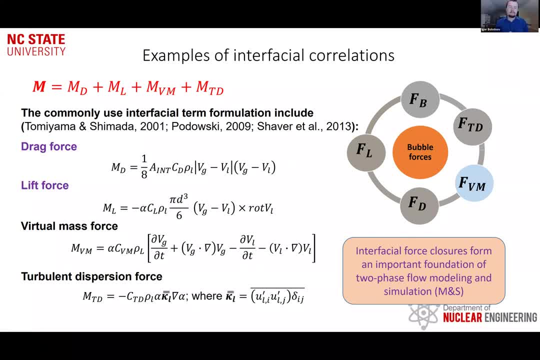 but often those logos ofекс�도, But often those closure laws. the coefficients are evaluation: patients are evaluated based on simplified assumptions such as, for example, having a spherical bubble, And there is a lot of interest at HGDR as well on how to improve. 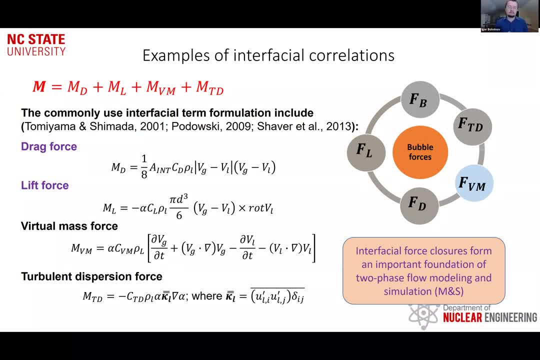 those closure loss. So the system level, multi-phase CFD for chemical engineering, you know you, for example, for bubble columns you can do CFD on a lot of interesting other problems which we have. Again, remember there's not too much nuclear stuff going on there, So 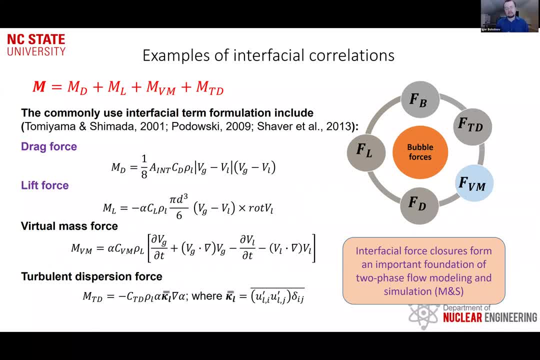 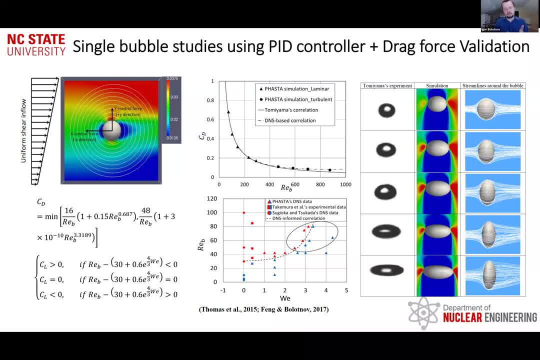 you know the, you know the um lift and drag efficient on a single bubble. So it was done by by my students in between you know um five to three years ago, based on the papers And um, this was one of the one of your kind of scope which were proposed. 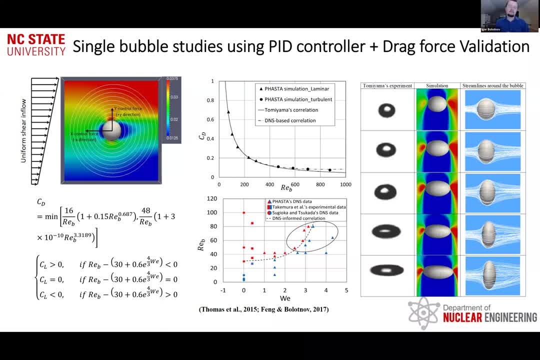 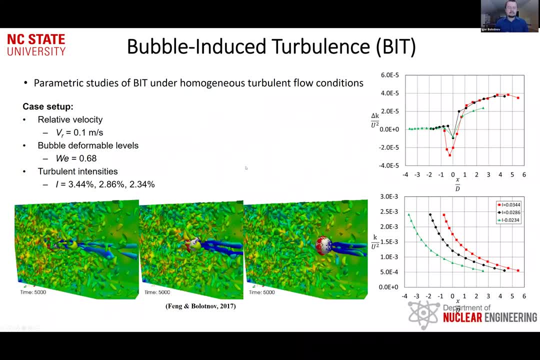 for the sabbatical state through to work closely with with bad colleagues to see how miss capability can help improve them on this Um. so this is another example, in a little bit more details, on bubble-induced turbulence. So when we perform those virtual experiments, 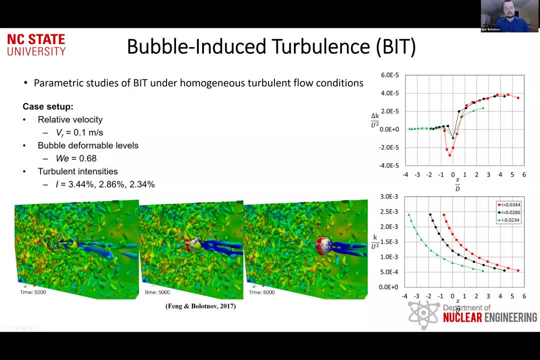 we can actually view the weight behind the bubble and we can visualize it. So those blue sort of streak lines, and this is turbulence produced by the bubble weight And you can quantify it. And then the question is, how do you take it further and improve the existing models? 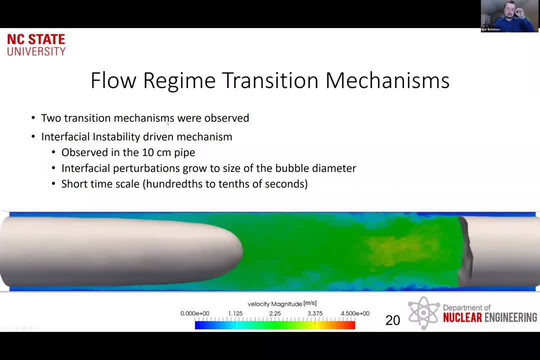 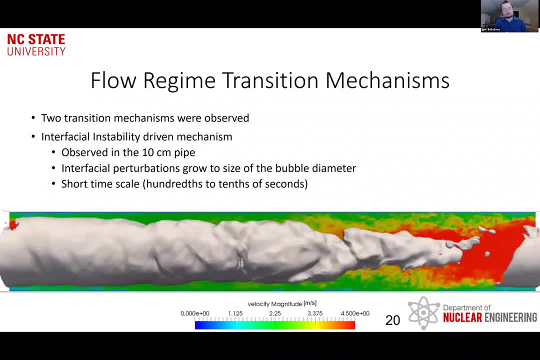 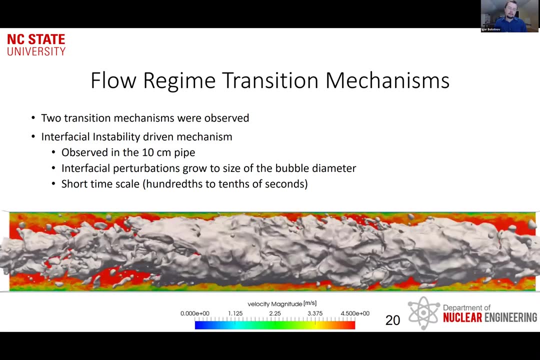 So a couple of examples of the flow regime transition. So I showed some schematics early. when you have higher concentration of gas in the flow. So there was a work by my student who finished in the spring And essentially one of the challenges become 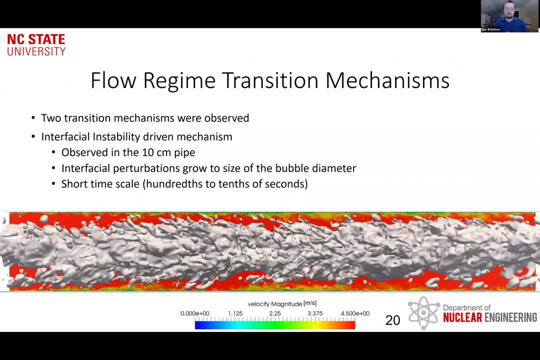 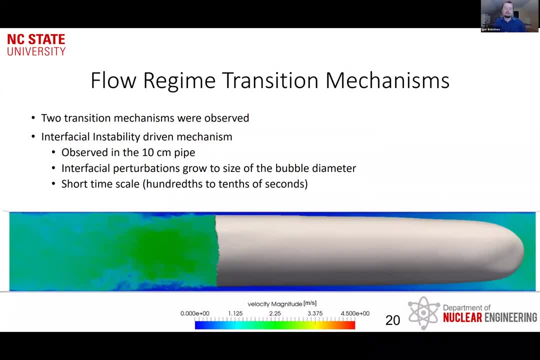 it's not only verifying valid data simulations, but also how do you process the results and how do you extract the data and how you make use of it. So this is another topic of our discussions with HZDR folks, And I'll mention a little bit what some of my students 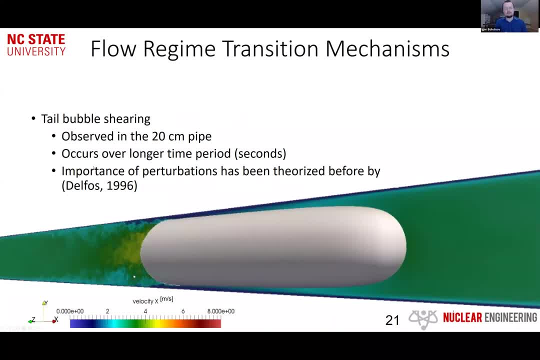 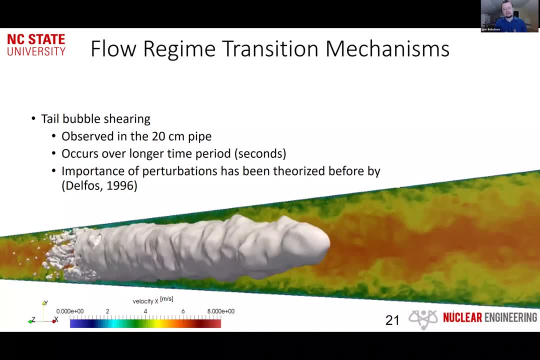 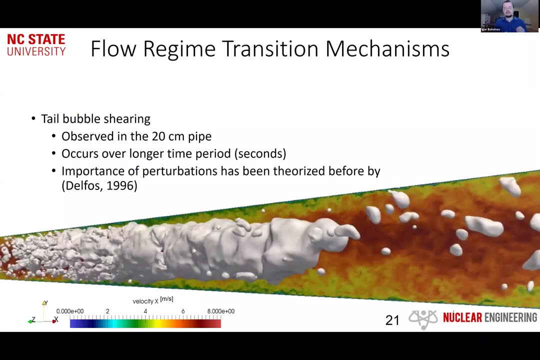 picked up and did So. this is a slightly different view of a different simulation too, So it's a longer domain, but it kind of gives you an idea what the capability of direct simulation is: direct numerical simulation to resolve the interactions and basically bubble large Taylor, bubble evolution. 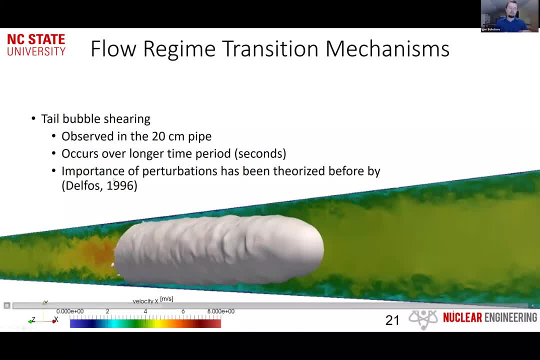 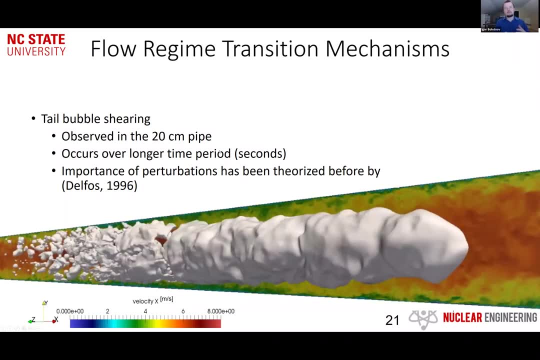 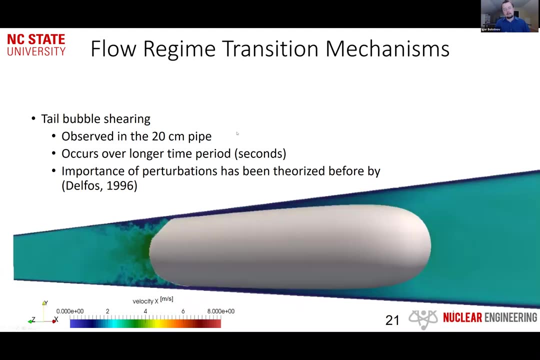 and interface instabilities to model the flow regime transition, And so this is very common phenomenon in BWRs, but not in pipes there, but basically in BWRs. you are going through those flow regime transitions to produce a lot of steam in the outlet of your core. 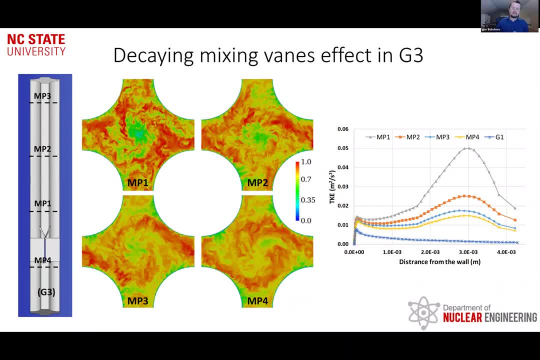 So a little bit more details again. just to emphasize, the code we're working with is capable of unstructured meshing. So we do deal with very complex domains and it's it's challenging, it's expensive, but it's also challenging to process the data. 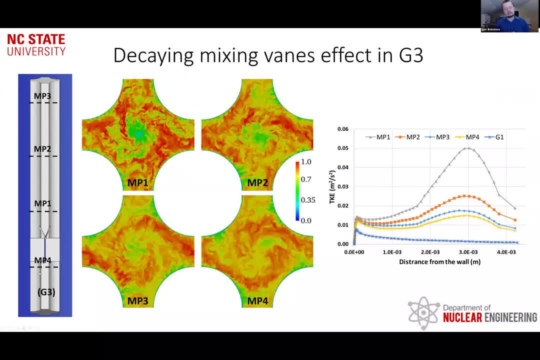 So this is a simple single phase, no bubble type of simulations, when we have mixing veins and spacer grids and we're basically evaluating the turbulent intensity in different levels. So for those who are familiar with some turbulence, so this kind of tells you that. 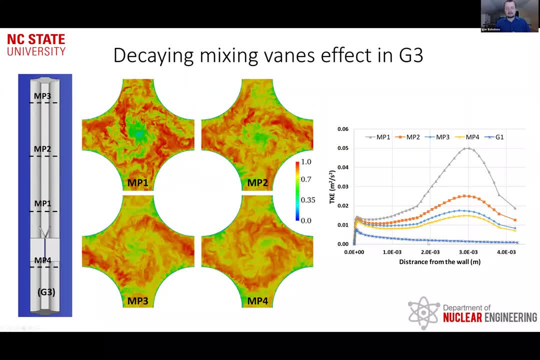 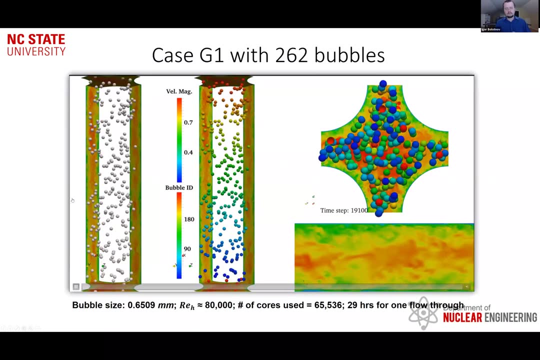 when you don't have any obstacles. so have a plain kind of channel flow or sub channel flow. you have very low level of turbulence. but the reactor structure really introduce a lot of two points and there is a good reasons for that, design reasons in the reactor. so this is just a short movie of bubbly flow and that. 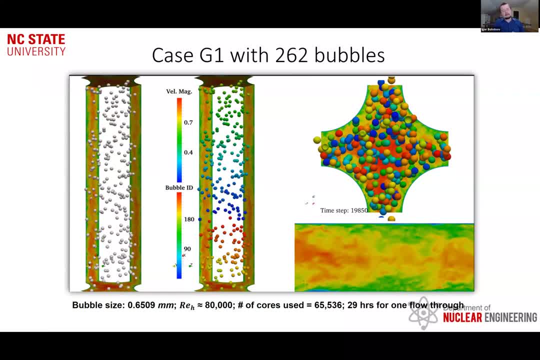 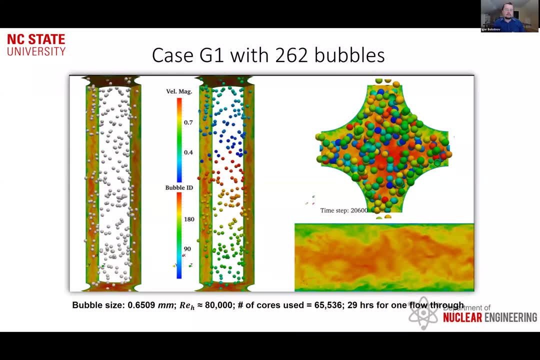 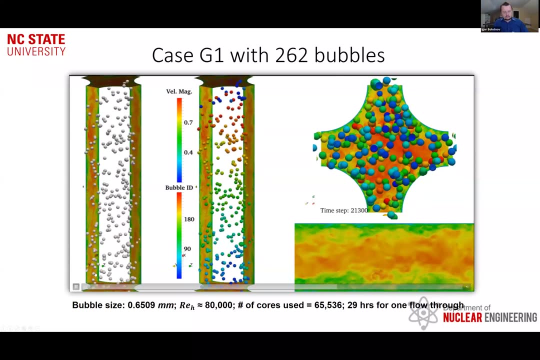 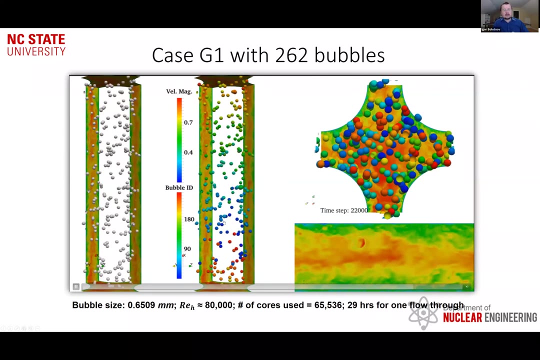 that's. that's actually another advantage which we discussed and analyzed during my stay at HDR, so it was done early, but the capability we developed early with castle project support is: instead of modeling interfaces, we, in addition to that, learn how to track individual bubbles, and this is easier said than 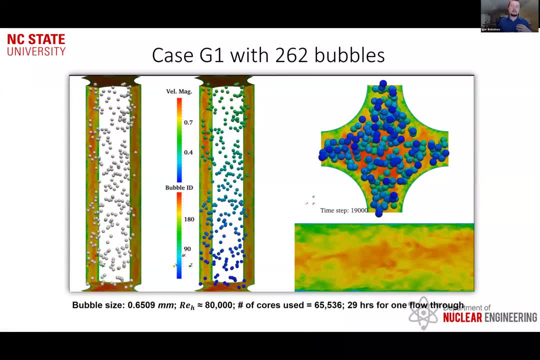 done. it took quite some effort, but, but basically, this bubble tracking algorithm which we introduced allows you to collect a new level of statistics for bubbly flow simulations and and really look differently at the model development. and that's what. that's what- one of the topics again which we looked at during 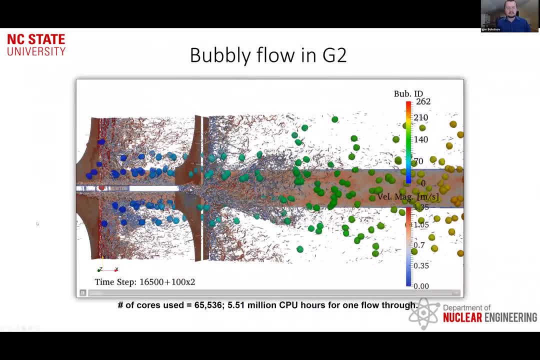 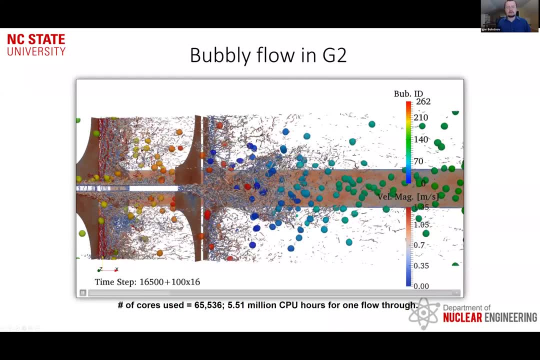 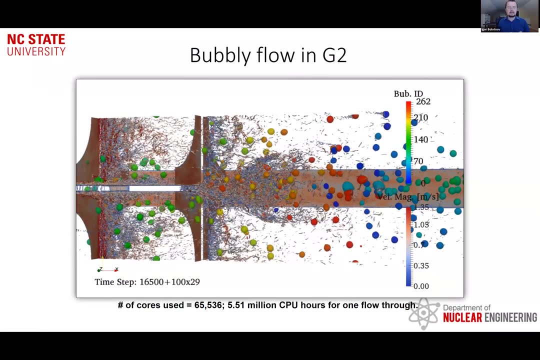 sabbatical. so this slightly different view of different domain. so you also have the mixing mains. now you have this bubble mixing and you visualize some, some turbulence levels. so one of the things which I also mentioned about the expense of your simulations: the domain sizes here are quite large in terms of 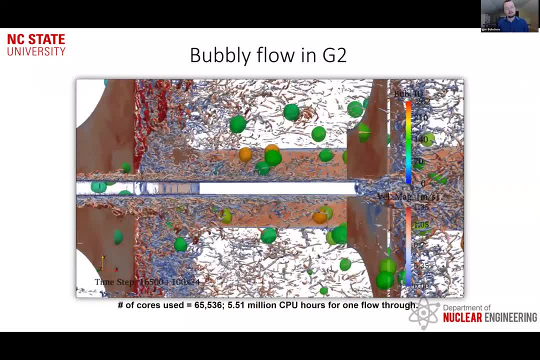 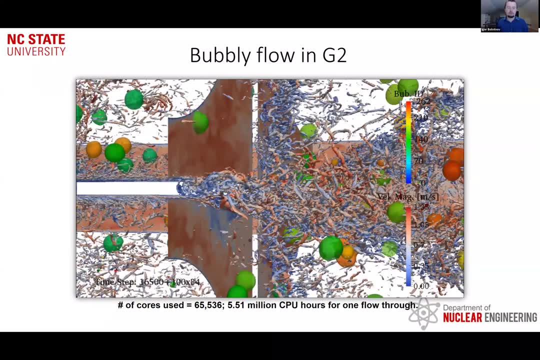 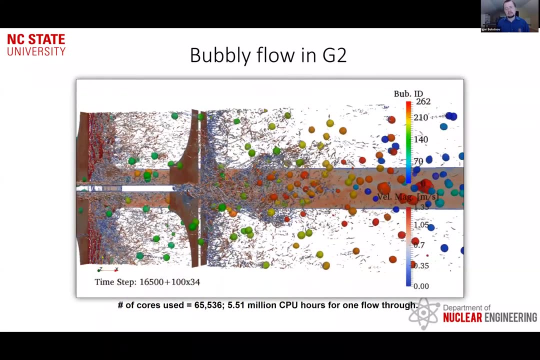 the number of degrees of freedom. so so this type of domain limits require about one billion finite elements or nodes to resolve these things. and so what we routinely do in my group, we apply for competitive allocation at national ops and we win this and we perform those simulations at 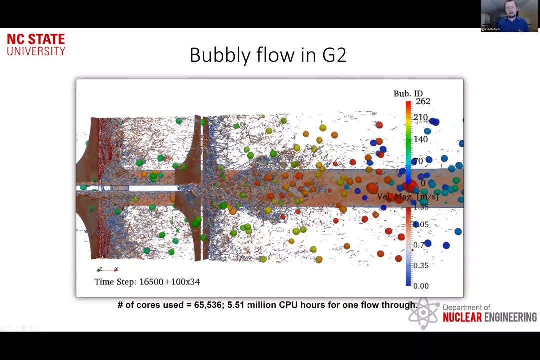 quite high computational cost. but again, the investment in the research at this level is is very important because, as the computational costs are being reduced, The hope is that the higher and higher fidelity and resolution type of simulations will be adopted by the industry as time goes on right. 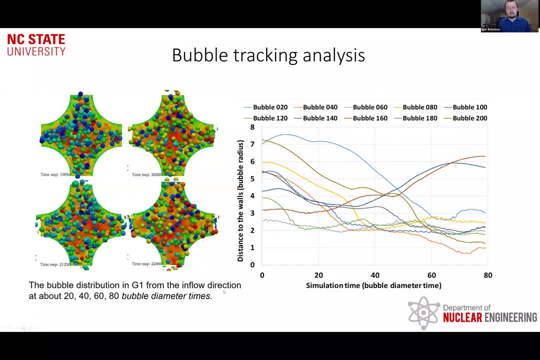 Because it becomes much more affordable. So just another small example about this bubble tracking So we can actually look at the distance to the wall which bubble and the lift force which I mentioned earlier for spherical bubbles in upflows. it actually attracts bubbles. 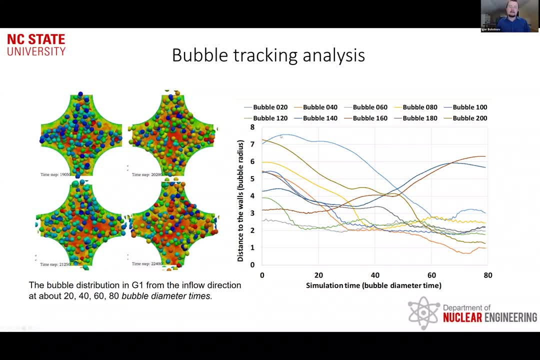 towards the wall And you can see that some bubbles would go seven radii away from the wall. Eventually it gets closer to the wall but some of the bubbles may kind of travel randomly and, I guess, approach the wall or go the other way. 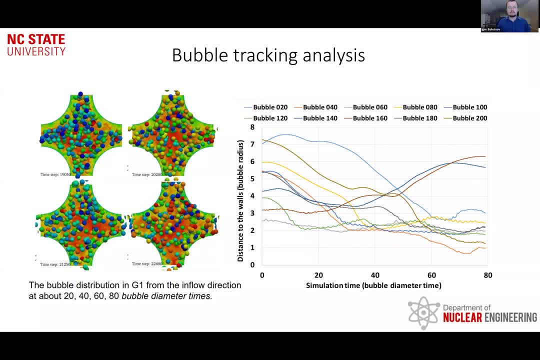 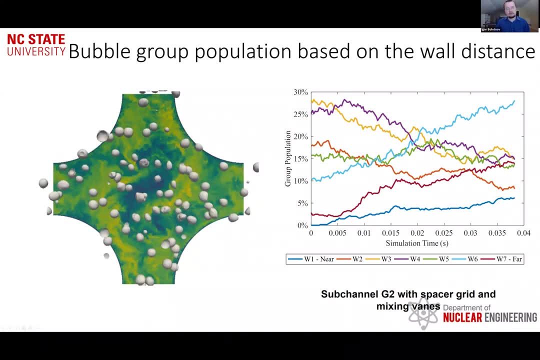 So this is a brief example of what bubble tracking gives, but obviously there is much more behind that, And so yet another view on PWR type of flow. So we have basically wake of the mixing vein, And so we have a wake of the mixing vein. 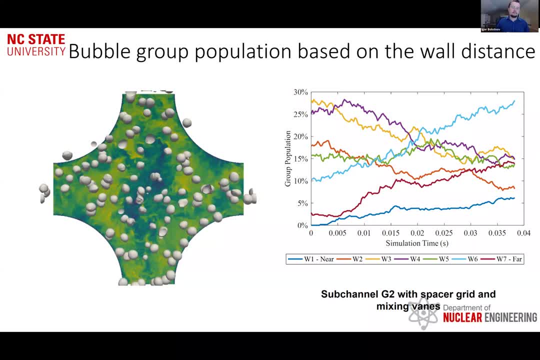 And so we have a wake of the mixing vein, And what is happening in the wake is now an interesting phenomenon. So the bubbles are light, they are from steam right. The liquid is relatively heavy, So mixing veins really create this centrifugal effect where the heavy liquid is pushed towards. 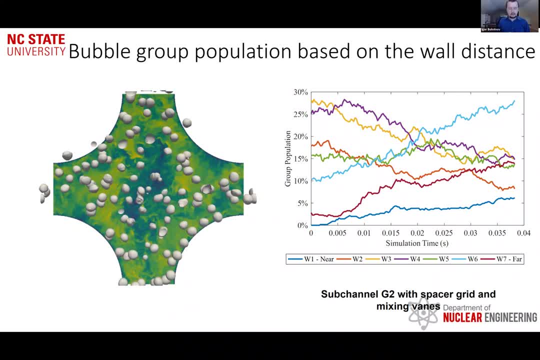 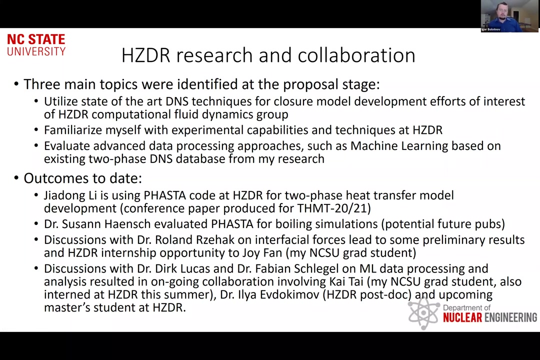 the wall. That's actually very helpful for prevention of departure from nucleate boiling in boiling channels, But also what that means is that it drives the bubbles towards the central line, So that's another phenomenon. Okay, All right. so a little bit to emphasize after this background on what we do in our research. 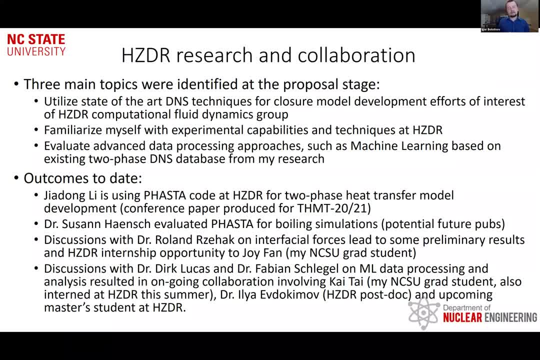 group. At the proposal stage we really look at the three topics for HDDR, And so the first one, as I mentioned, using DNS to develop closure models which are of interest for HDDR. Then I wanted to really get a little bit hands on with experiments, so I never done experiments. 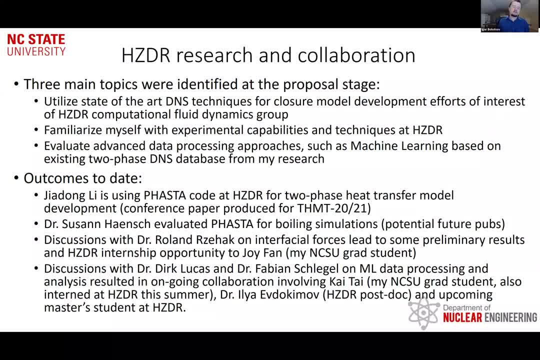 So I think that was my first step. And then I wanted to give a little bit of a hand on with experiments. So I never done experiments, uh, before in my career. so i wanted to, and and i think we did some of that and we hoped for another three months, also to. 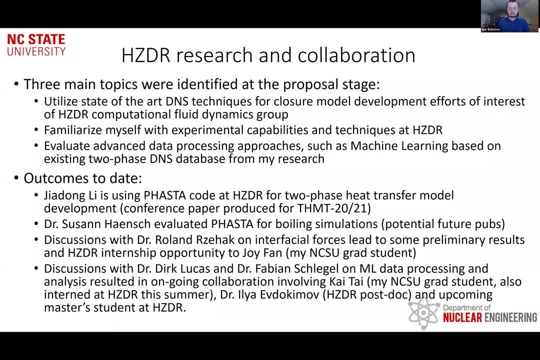 to get a little bit more exposure, potentially, but not much, but at least kind of interacting with and discussing. actually, discussions are very, very useful because you really have a different perspective, uh, from the simulation point of view, experimental point of view, and you know when you ask more questions, you know, you know. 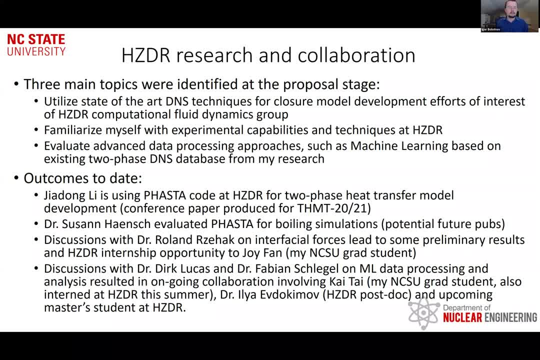 more and more so. that was very, very nice multidisciplinary interaction. and then, uh, look at this, data processing approaches. so that's that's one of the um, one of the major issues- that the more data you generate, you know- especially if it's validated and high quality data- uh, the harder it is to process and to 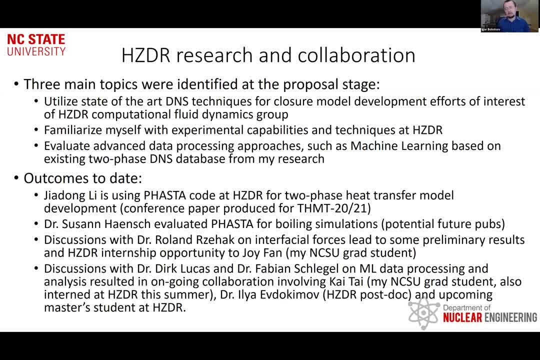 understand right. so if you have a single bubble, it's it's kind of easy to figure out what's going on. if you have thousands of those, how to make sense out of it and extract as much values as possible, that becomes more challenging. so one of the 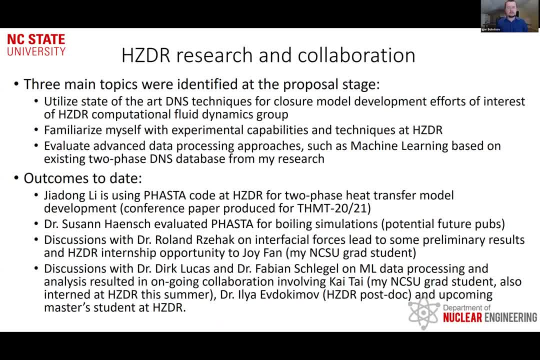 students at hcdr actually picked up my code and and we were looking at some interesting two-phase heat transfer model development and, uh, we call for it a couple of papers. one of my students, kai tai, and submitted for um, what is it? i'm trying to recall the thmt conference name, but but anyway. so the 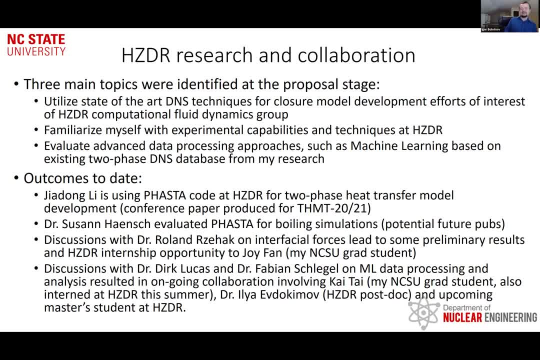 conference as well, was planned for uh for uh, summer 2020 and saint petersburg, so it would have been already presented it, but they pushed the conference to 2021. we all know why, uh, uh, but but yeah, we have a time to improve the paper, i guess. 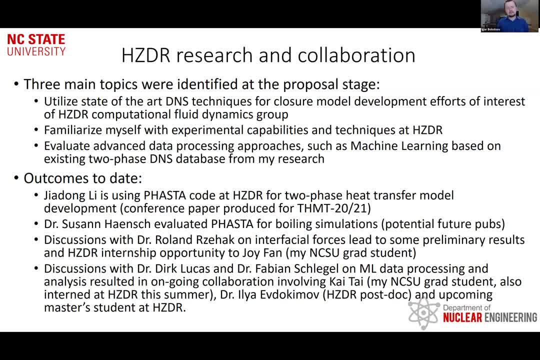 in this effort there is a postdoc, dr suzanne hange. uh, she looked into the boiling capabilities of of pasta as well, but then she got on our project. but maybe hopefully again after that experience it, it will be picked up eventually and- and that's one of the sort of um issues, uh, of of of you know, being on. 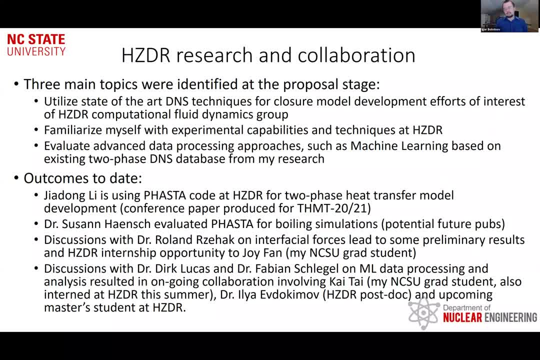 sabbatical because, um, um, essentially, uh, while everybody is happy to host you, interact with you, uh, as, as you, many of you may know, in the end of the day, it's also the money issue, in the sense that, while sabbatical, or fellowship, does support my time, 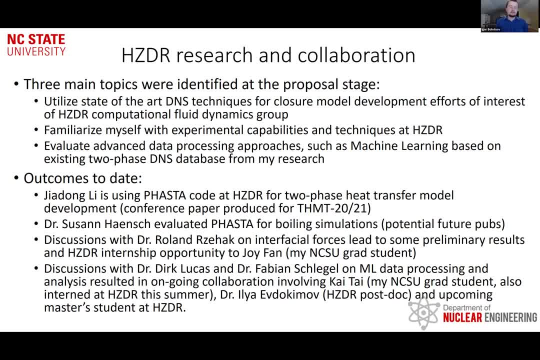 it doesn't really support much more than that. so, essentially, whoever you're interacting with is is, you know, taking time away from other projects, right? so so there is no, um, very small support for like equipment and and um, some some, i guess, desk space and whatnot, which which, uh, foundation may. 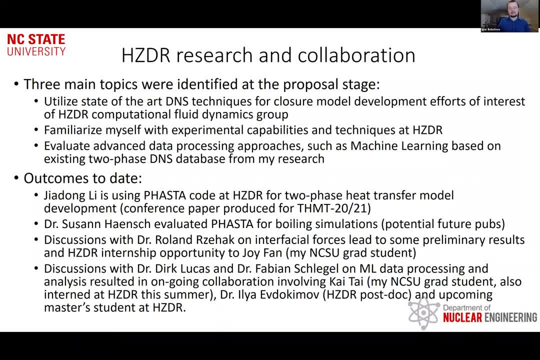 may pay, so so. so this is- this is still sort of a um, a special situation in this scenario, but um, we had nice discussions with uh, dr uh, roland uh and joy uh, who is who is in my group, um, and he in this seminar, um, so she had an opportunity to to take a virtual internship, so that that's a. 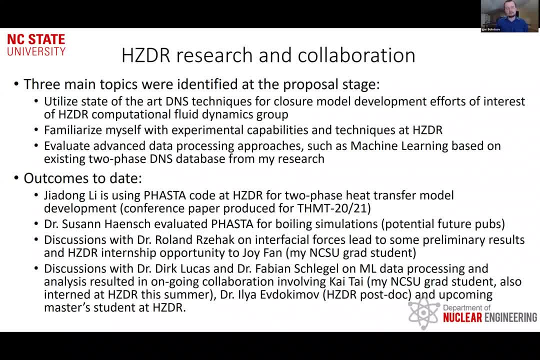 that's actually actually the sort of the advantage of of the covet situation, i guess, because going to internship in germany would have involved otherwise, uh, much more effort right than doing it remotely uh. so she looked at these interfacial forces, uh evaluation, um, and we had some nice. 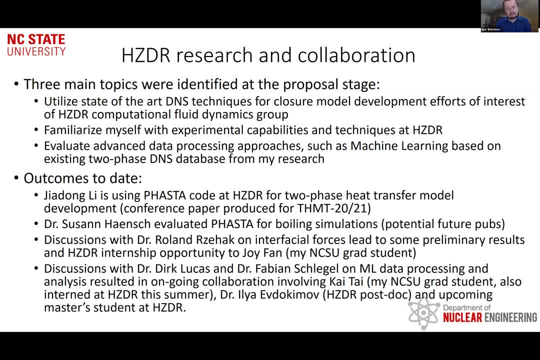 discussions with roland on that, um, and then, uh, dirk lucas was my main host, and then we had a junior um researcher there, but well, young researcher but not too junior, i'll say um, and we talked to, uh, we had an extensive discussion on data. 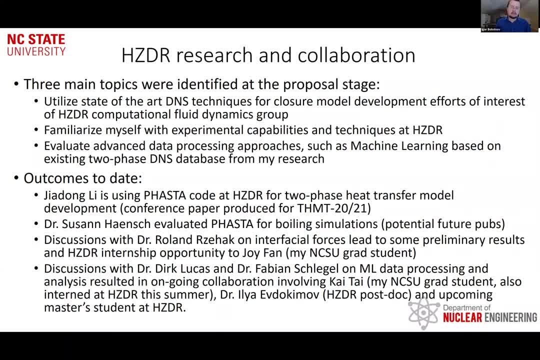 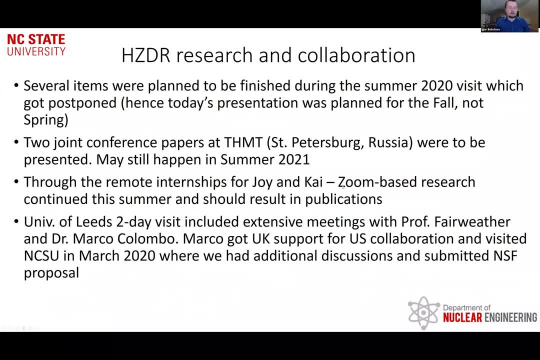 processing, how to apply machine learning to those things, uh, and then later hired, i think after i left, uh, ilia, if they came off and it's kind of getting picked up, and then kai again also took this internship, uh this summer to to move this forward, okay, so, uh, yeah, i'll try to. 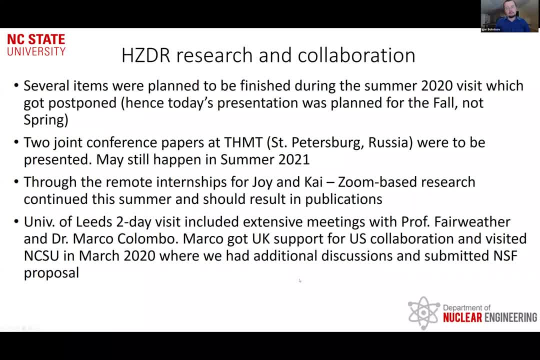 move quicker because i have more slides in time, i think, and and my voice is not getting better. um, so, basically, um, again, we had more activities planned for summer. hopefully will happen in 2021. we'll see. um, i mentioned about the marcos visit that was. that was very nice. we actually 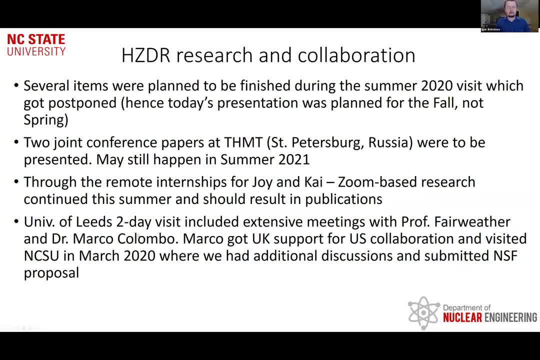 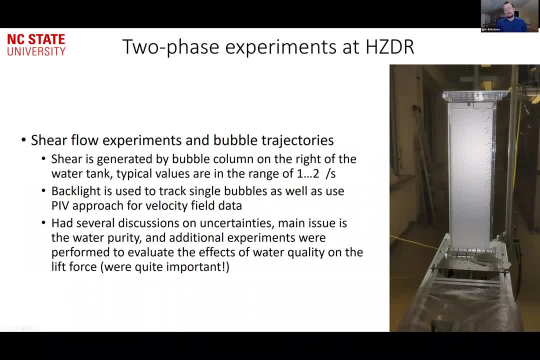 submitted an answer proposal with him and hope for some future collaboration as well. um, so, these are some, some examples in terms of experimental exposure. so, uh, the lift force which i mentioned and one would like to evaluate, uh, precisely occurs in shear flow, so it means there is a sort of gradient of the 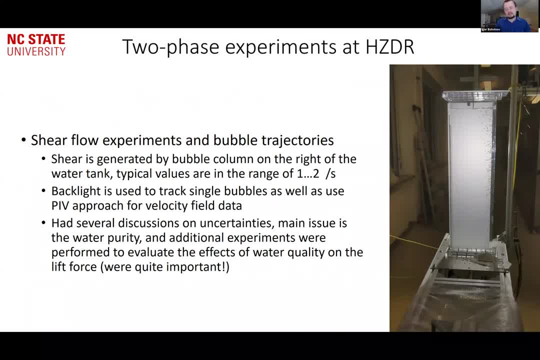 liquid where the bubble goes through it. so the very kind of fairly simple tabletop facility which azdr has- and they have actually have a huge experimental facilities which are world known- but this is a very sort of a toy which we designed but it took them some time to figure out how to do it right. 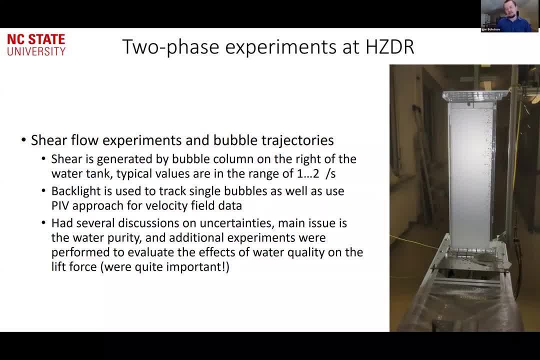 so we have a sort of bubble column on one side, and if they do it carefully, they do create a very uniform and nice shear of the liquid due to the recirculation of the liquid which is driven by those bubbles, and and so we, then we inject a single bubble here. 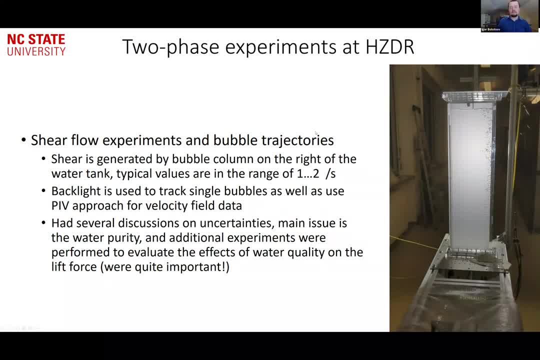 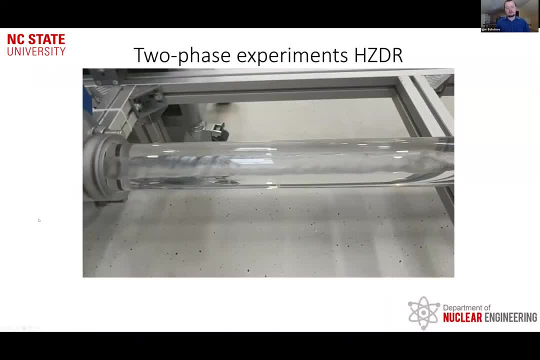 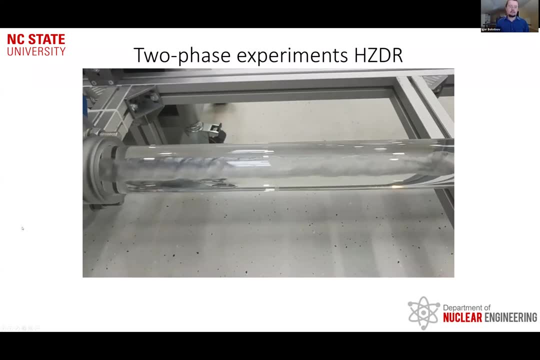 and we watch the trajectories and maybe do post-processing and we figure out how hard the bubble was pushed to one side or the other. uh, this is a somewhat larger facility which i didn't wasn't really involved, but uh, this is sort of an industrial project which we had and the idea was: 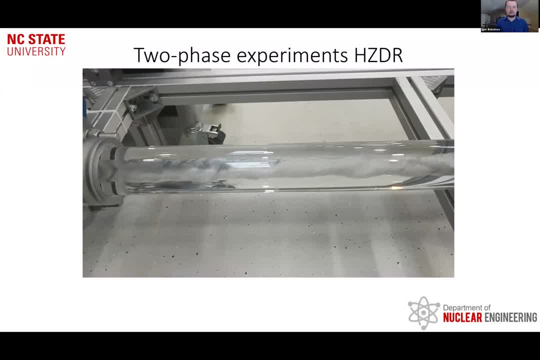 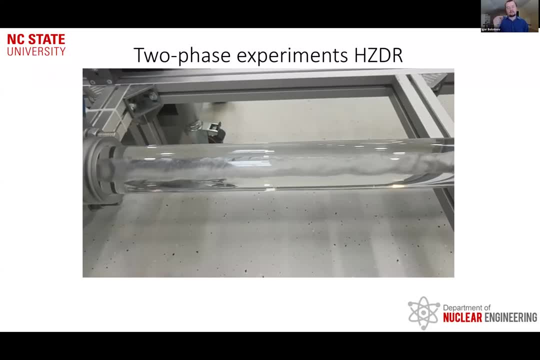 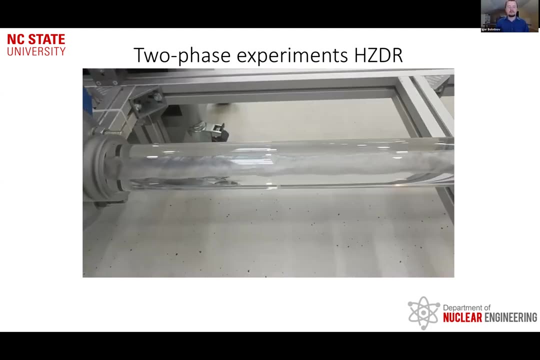 to separate liquid from gas and they would actually, um, have this uh strong swirl in the two-phase flow and then they would have a suction pump right in the middle of the channel and you can suck out the whole uh air or steam, and so basically that sort of a flow separation kind. 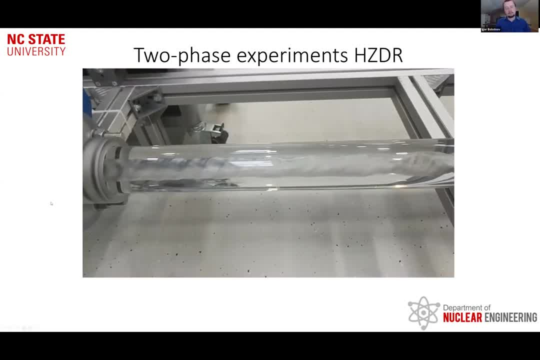 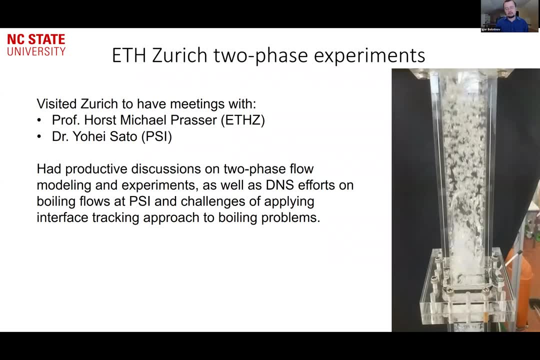 of design. so it was kind of interesting during one of the tours which i took, uh when i visited, uh uh, professor misha prasser- so he's a quite well known- is also in the ath suric. so so i took some videos with my cell phone. this is a slow down video of of a 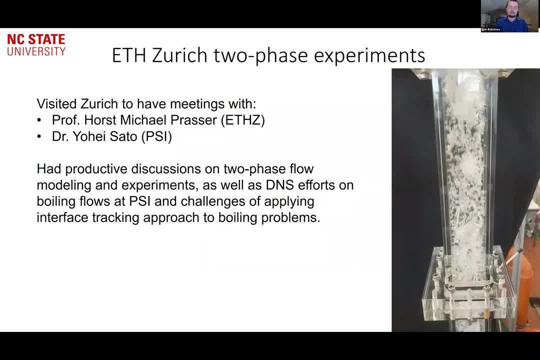 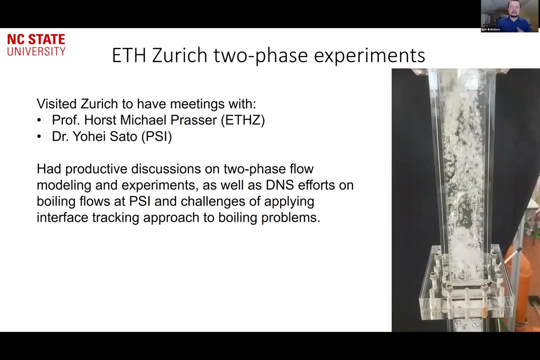 germ turbulent flow in a sense. so you have those taylor bubbles going through and then there is a- i'm sorry- and there is essentially um, uh, mixing, mixing between the small bubbles and bubble bubble, uh, coalescence and breakup, and these kind of things, uh, also, uh, 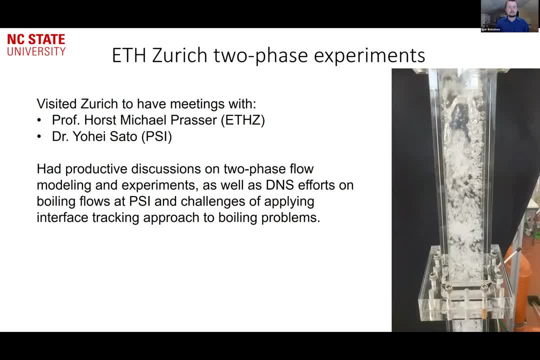 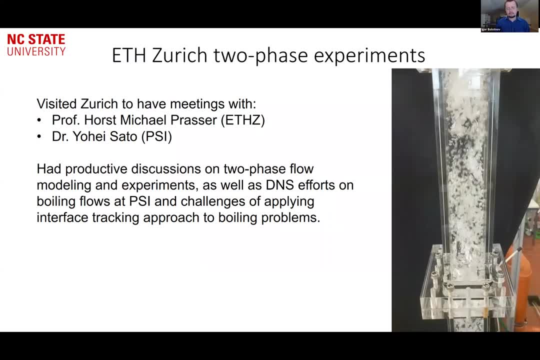 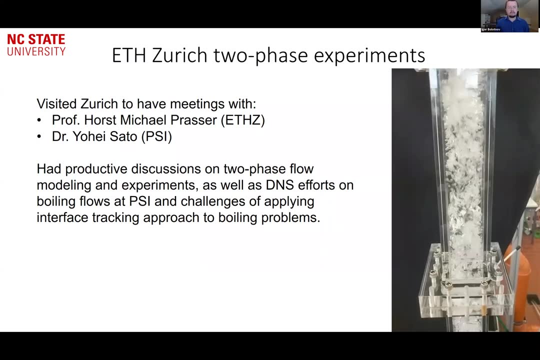 doctors. arekel, he, he's doing some dns or boiling flows at psi. so psi is a sort of national lab at the th zurich university. they are actually a little bit apart. um, uh, what i remember about zurich, i mean it's a nice city, but but the um the cost of living there. 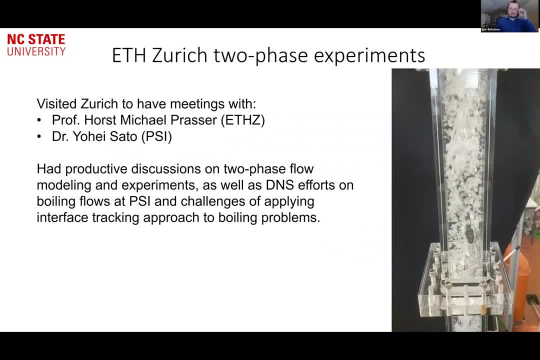 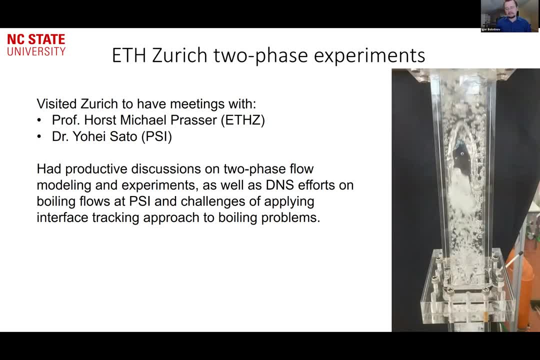 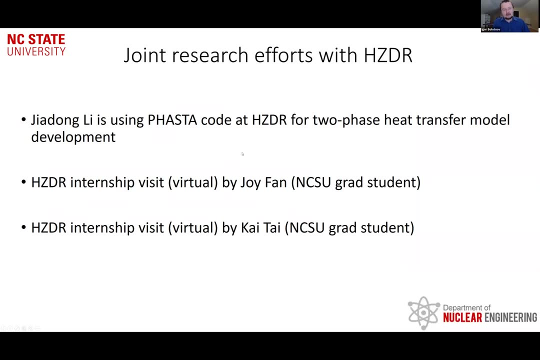 is is huge. and then if you look at the ratings, it's, i think, number one in the world. so, um, just going in grocery store, uh, the price is something, Anyways. so so these are. these are things which I kind of mentioned and what I 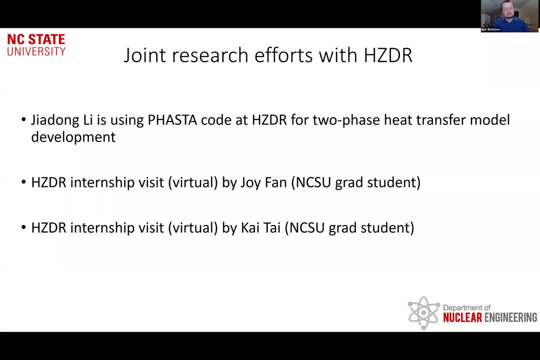 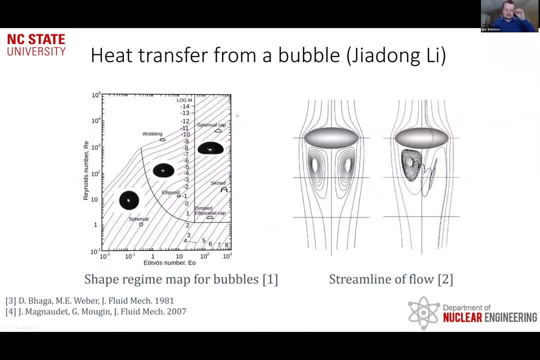 want to briefly review in the next maybe 10 minutes. no more than that is is a little bit more details. So Jadong Lee. so he's a student again at the HDR. So so look at the heat transfer around different bubbles. 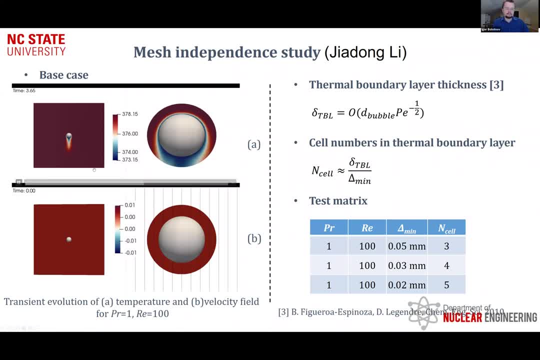 And what we did with with our code, is essentially look at a perfectly spherical bubble and to see how the heat transfer occurs, to verify that, that the code can do. that, I think, And the tricky part is that the correlations exist which are pretty reliable for spheres. 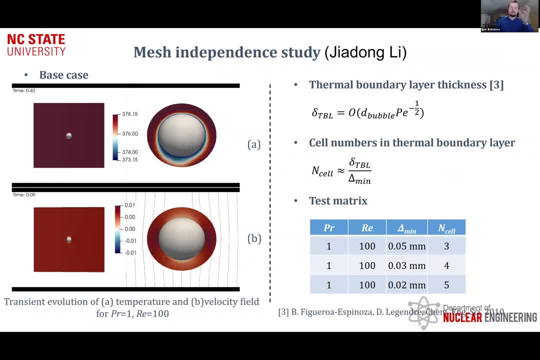 So if you have a sphere, you know what happens in terms of heat transfer And it's not uniform, right? So you have different boundary layer thickness on the top of the sphere versus on the bottom, And but then nobody knows what exactly happens. if this 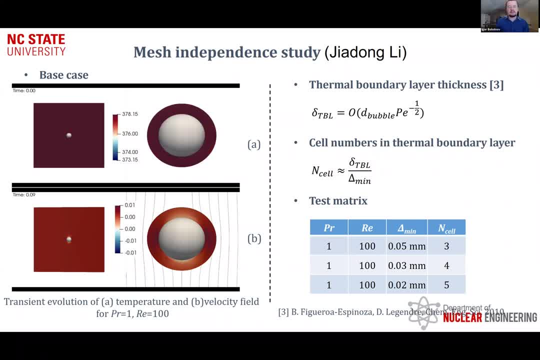 the bubble becomes non-spherical, which the larger bubble are typically non-spherical. So so the so this is a sort of two-step project And I think he completed the first step and probably still working on the second. The first step was to make sure 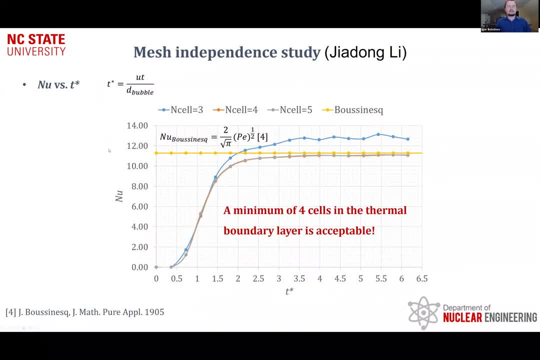 that we can properly predict the Nusselt number which characterizes the heat transfer coefficient, and find the correct resolution of the mesh to to, to, to evaluate it for a spherical bubble, because we know some analytical solutions on that And so and but then we 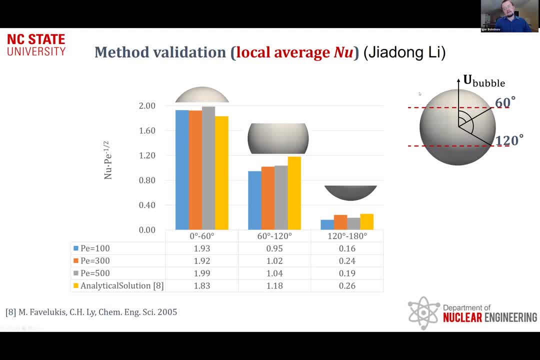 one of the things which we decided to do is to look at the in order to have a better predictive capability, to split the model into sort of different parts around the bubble, So what happens at the top of the bubble, on the sides and at the bottom. 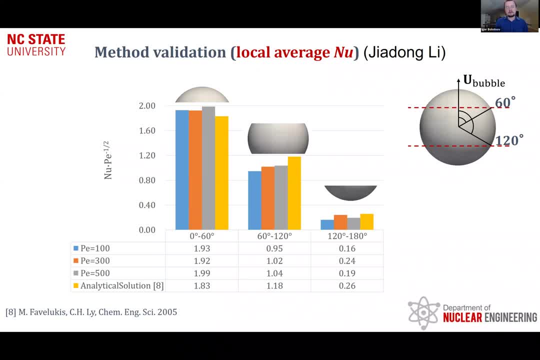 and and and then use additional numerical experiments to look at the spherical or non-spherical bubbles and see how those heat transfer correlations around different parts of the bubble will will will basically behave right, And then you can develop actual model. 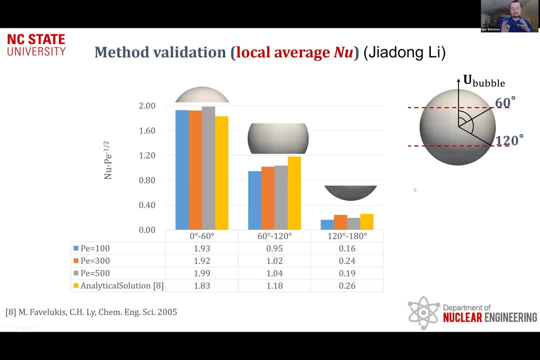 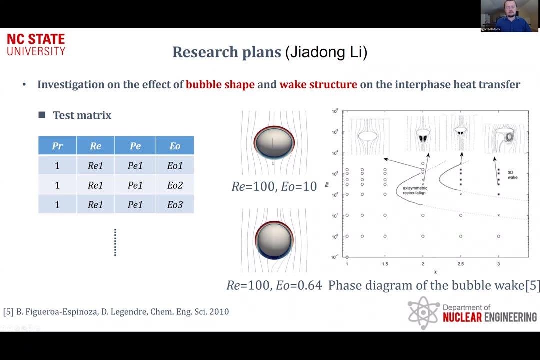 which would be much more reliable because you're actually looking much closer at the physics versus empirical correlations or or solutions which are only limited to to the spherical shape. So there are some, some examples here: when, when you, when you create the non-spherical bubble. 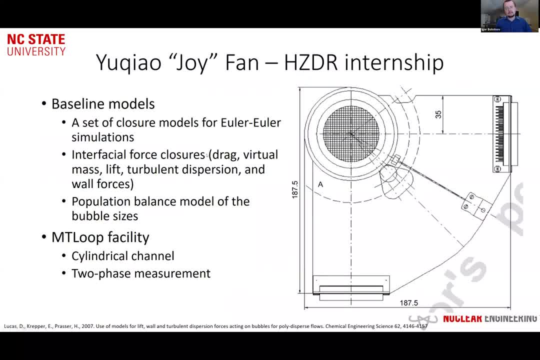 Um and and again. this is ongoing work, So the other effort. so, Joy, I picked a few slides with what she presented early to our group a month or two ago, and and they, I think, and and the idea was to to improve the so-called baseline model. so baseline model and hdr, we chose. 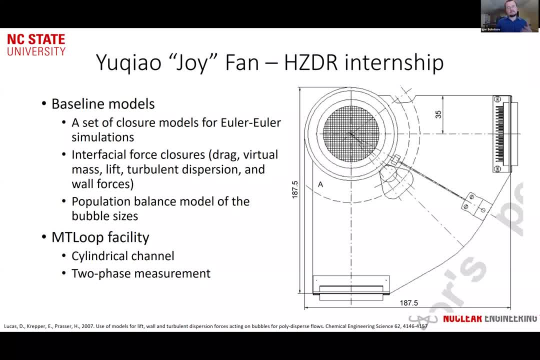 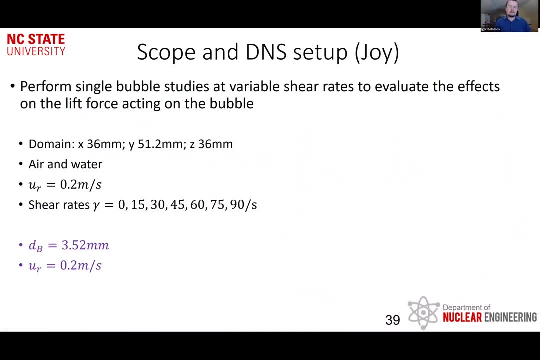 that name. but the idea is that again we have a set of forces and they have a bunch of verification, validation cases and they want to make sure that this model, sort of um, gives a good predictive capability for a wide range of conditions and that we're interested in in terms of the the 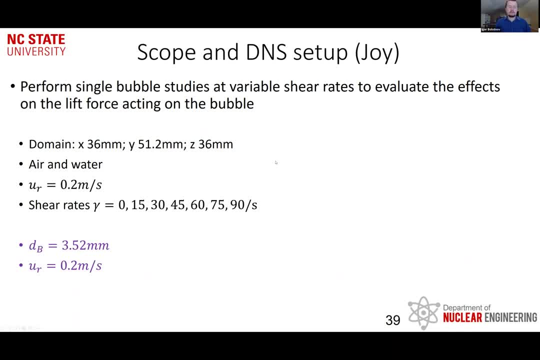 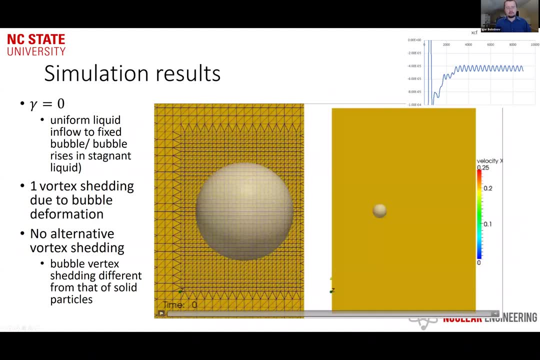 work scope for joys, as to what happens if you increase the shear rates- and higher shear rates are very important and we looked at it at some point in the past. uh, and and enjoy did a few simulations and i think she is yet to complete uh or update the report for them. i think, yeah, i mean. 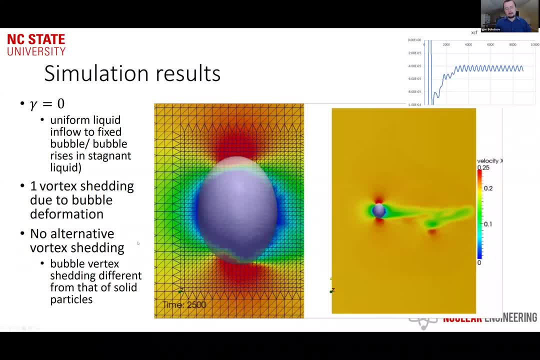 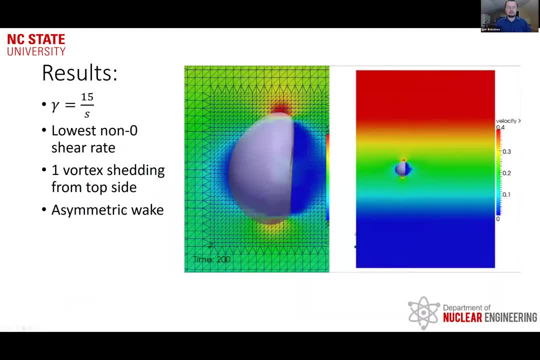 she did the report, but, um, but she was busy with our stuff, um but but essentially, uh, looking at different conditions and different shears, and, um, so this is, this was no shear. and now you have the different conditions in different shears. and so this is, this was no shear, and now you have the. 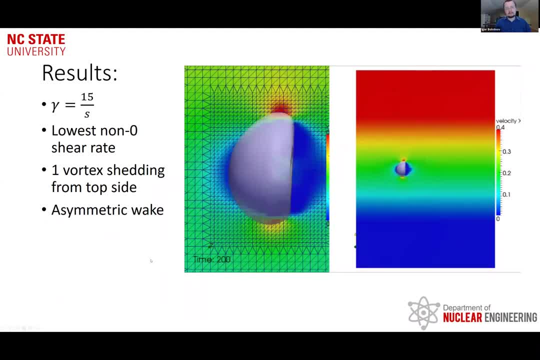 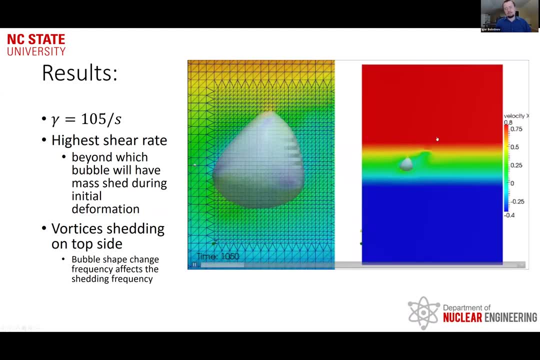 shear of 15, one over second, and then on the next slide, um, you have shear of 105, so it's a very high shear flow. so you can have sort of a turbulence being produced and at the bubble uh top side, and then there's even some sort of a backflow going on beneath the bubble uh. so physics fundamental. 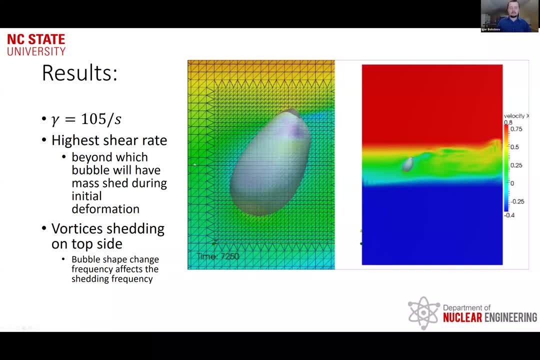 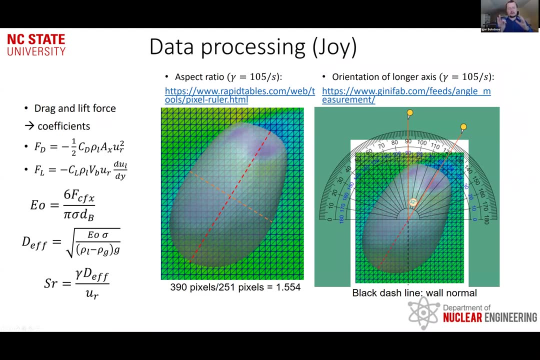 physics changes a lot, um, when you, when you really tweak the, the bubbly flow uh conditions significantly right so so it's important to capture that in the models in order to have predictive capabilities in in the variety conditions, uh. so one of the things which she did, she'll look at the bubble inclination and then then another trick is that when you resolve, 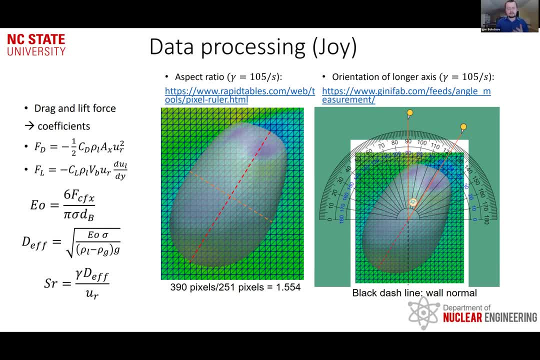 everything in a, in a um, with a high resolution type of method you have to really pick and choose some of the parameters which could be resolved with with a coarser sort of uh approach, so in game a course approach, when you have only bubble concentration, you typically would assume. 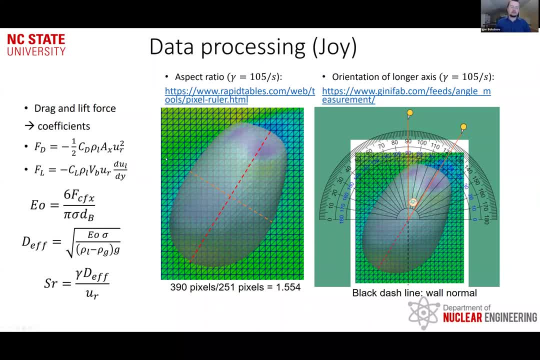 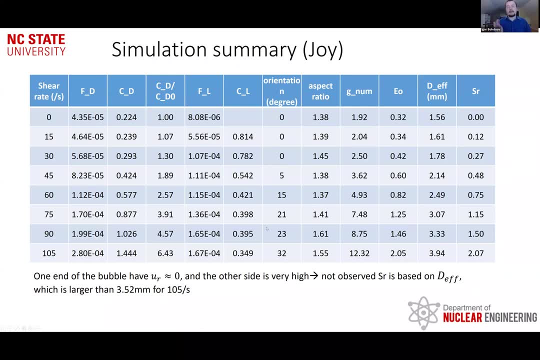 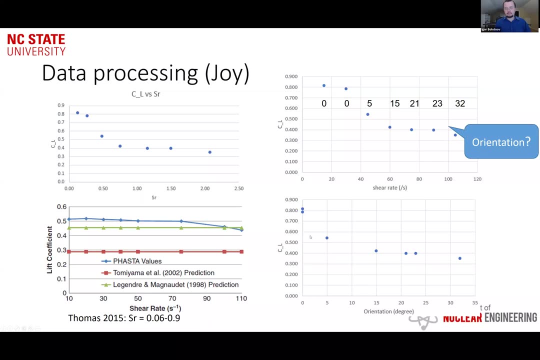 the average bubble size. so so, so more details would require additional modeling, so, but here it was some some uh dependency of the drag coefficient and lift coefficient on the degree of orientation and aspect ratio of the bubble. so it was a bunch of cases which you performed. they kind of summarize that, um and then and then there's a dependency of this. 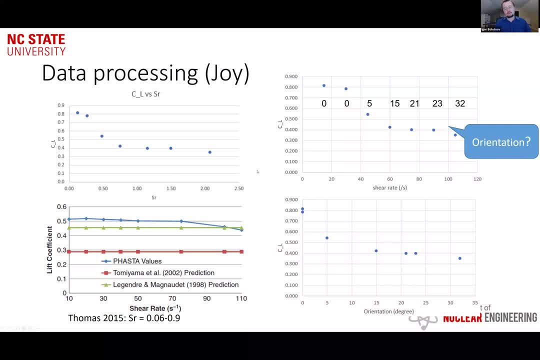 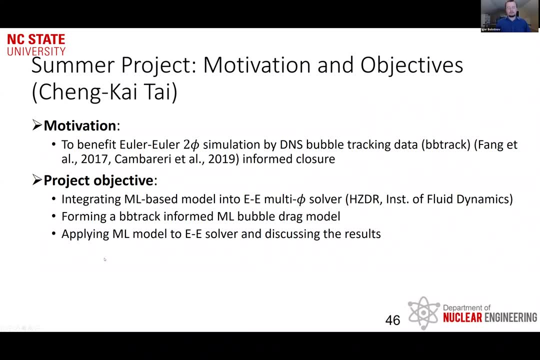 lift coefficient, on on on those parameters. so i'm not going to go too much in detail here. so if i, i'm just going to call it a on line, set below, if you have any. hi, hi, exactly, and so the first thing that we just talked about was one, the first thing we saw in 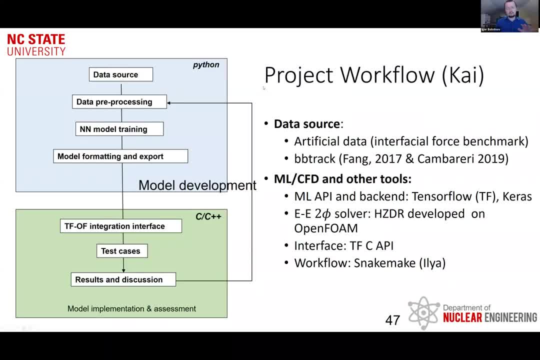 the first turning point to in this браслет with um, the training through ap haven. we running into zolder line training toateful Leslie uh test. we ran into that um on the the 1996 and and um 2013 data processing from- in our case it was DNS or first artificial data so we can generate. 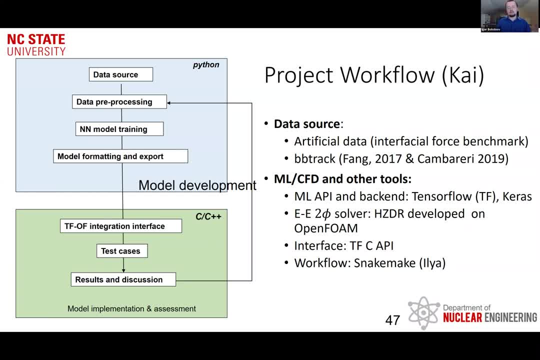 a lot of data, simply, but we know the correct answer. but then the actual data from our public flow simulations and then connected to the solver, to the coarse grid, solver open form, which is well-known and highly used, and basically having this framework when you. 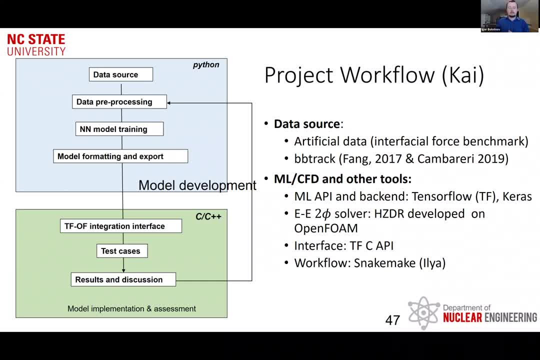 feed the data and you have an improved model pretty much right away. So I'm trying to see if Kaita is here or not, but basically I think that was a very, very nice start to this methodology and again, the idea is that as one runs, more experiments. 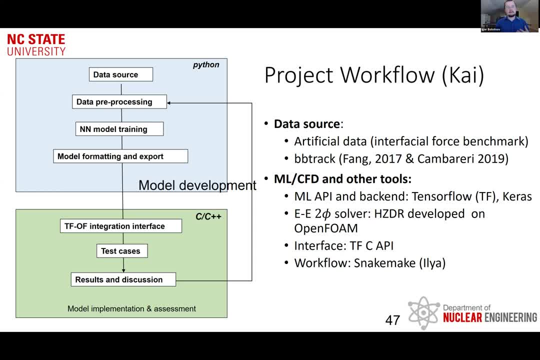 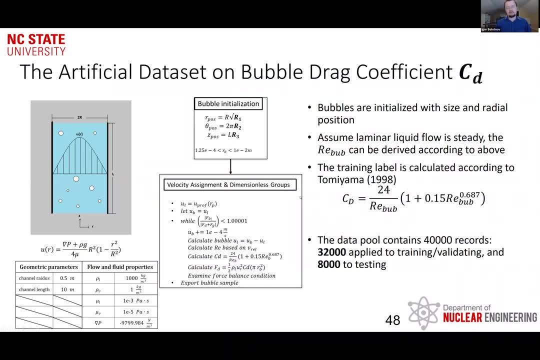 or more DNS simulations, which are expensive. how do you quickly process the data in such a way that you model on your industry level type of code? So give the word, okay. So I think that was the the general idea, And so there are some details here on the artificial data generator and how can we verify. 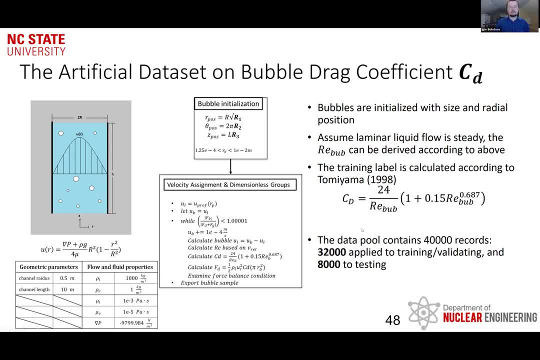 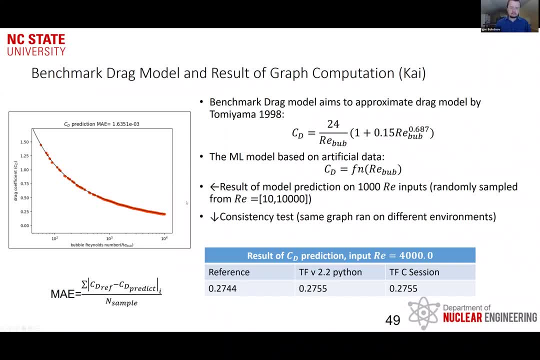 things to ensure that we get out what we put in. So that was the main purpose of that And if you have some verification of that. So basically, we read points what machine learning learned from the artificial data and the PCI black line is what it was supposed to be, and then he applied to some actual data. 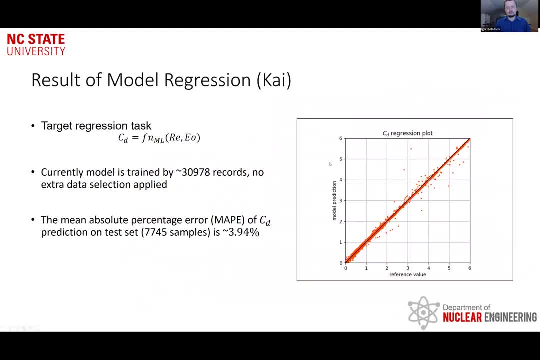 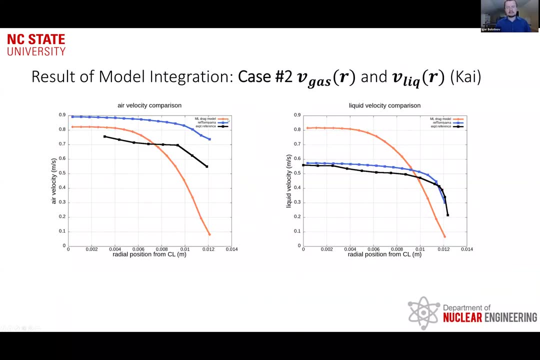 and again, not going to go too much details due to lack of time, but when he did some regression approach to basically evaluate the drug coefficient as a function of randomness and atlas numbers, deformability of bubbles, based on the actual data, and there are some results here, but i think there's, uh, well, yeah, so yeah, room, room for improvement there is still so so we 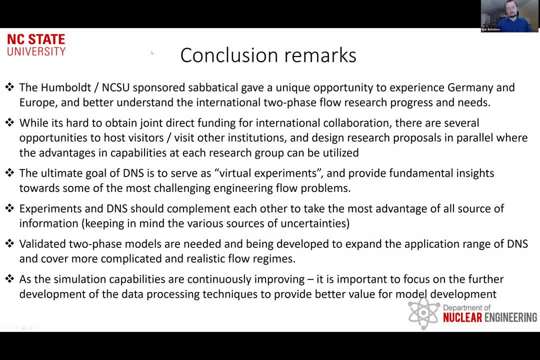 uh, work in progress, uh, basically all right. so to conclude my talk, um, obviously you know, sabbatical is nice. it's very nice, unique opportunity for me and my family as well. so i i traveled there with all my kids and my wife. um, it's also very interesting to kind of experience firsthand. 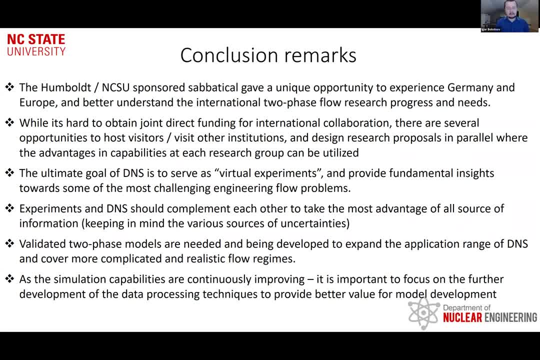 how, how research uh uh is is done international, in in our countries, basically, and uh, and what are we needs of that? so that that's also very important. um, direct joint funding for collaboration is typically hard to apply because if you apply to us funders, they don't want to send money overseas. 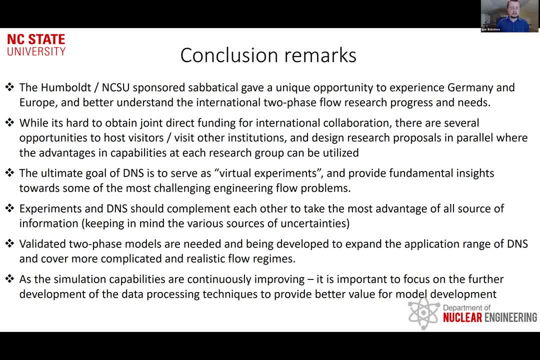 but uh, there are potential opportunities in the future to actually host visitors or visit yourself. so for example, as a part of humble they have a postdoc program for germans to go overseas, so potentially i could host a german researcher as a postdoc in my group. um and and and humboldt. 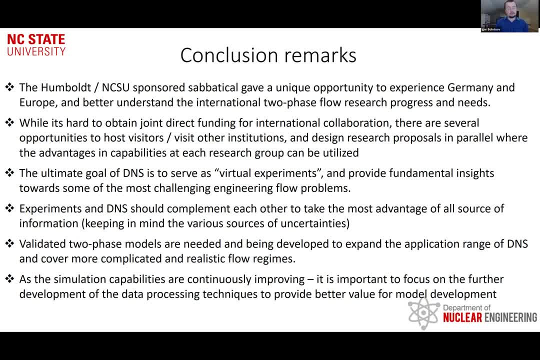 actually would well pay- not all of it, but they would pay two thirds, so i would have to come up with one third, but it's still a very, very good opportunity. um so, with dns again, we do so-called virtual experiments, but it has to be verified and validated for the conditions where we applied. 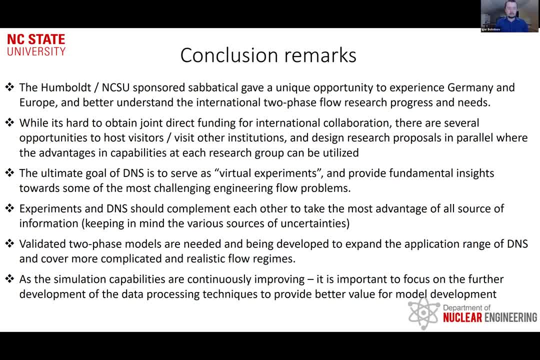 uh, learning how to complement experiments in dns is important as well and, uh again, the, the improvement on simulation capabilities is, is, is, is moving forward quite quickly, so so data processing is important, so basically taking taking advantage of that. um, just checking. so the last is the acknowledgements slide. 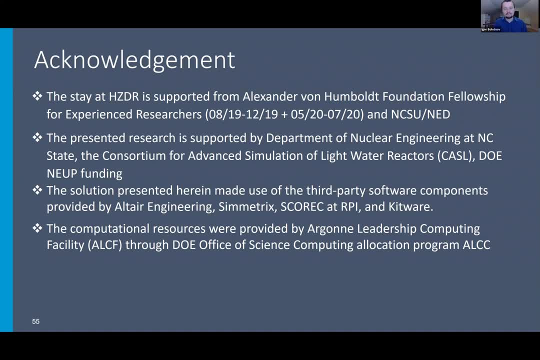 um, i'm not going to read that through. thank you for your attention. thank you very much for uh, for an awesome talk and for some great reminders of how much fun it is to travel. it's been a pleasure to talk to you. thanks for this session and thank you for your attention. 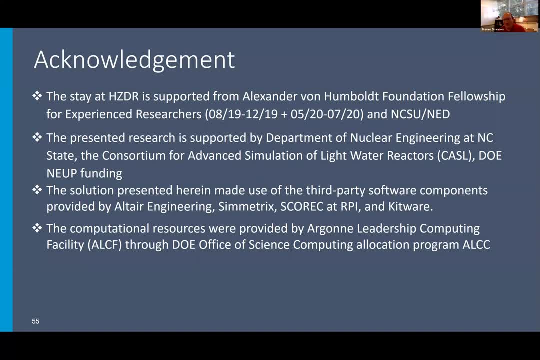 ever get to do it again. um, questions from the audience. please either free. feel free to please raise your hand and i'll unmute you, or um or uh, or feel free to post something in the chat. give everyone a couple seconds to type away if they have questions. 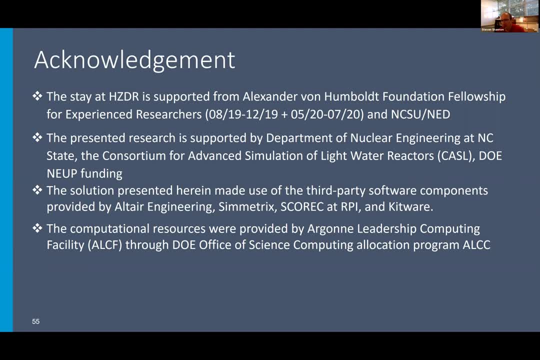 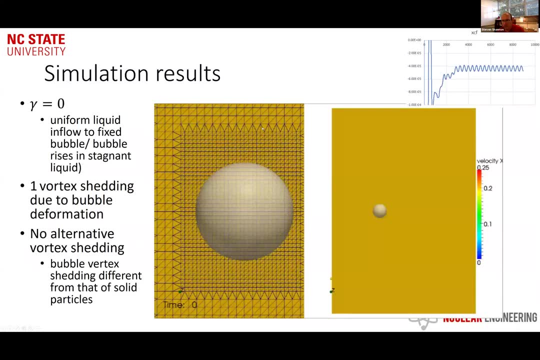 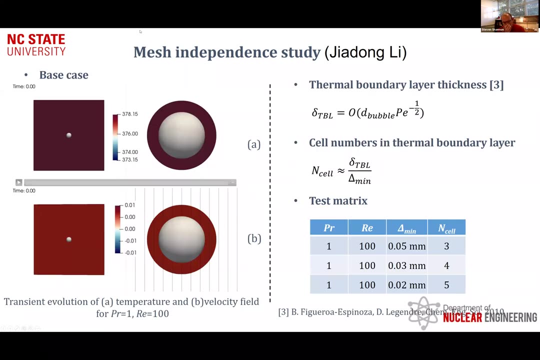 um. so one question i have is how much? how much of this? you mentioned that you use a lot of the um you apply for a time on the big, the, the, the, the big computers in the doe labs- um, how much of this has to be done there versus? i mean, how much of this can be run on like nc states, hbc or just smaller? 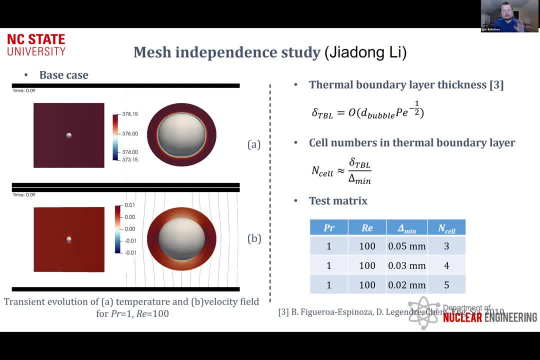 so so when we're talking about those sort of single bubble studies- so maybe a few bubbles um, uh, we do a lot of uh work on. we have our own cluster which is like 600 cores, um which which which i managed to get from some nrc faculty development funds early in the day it will. 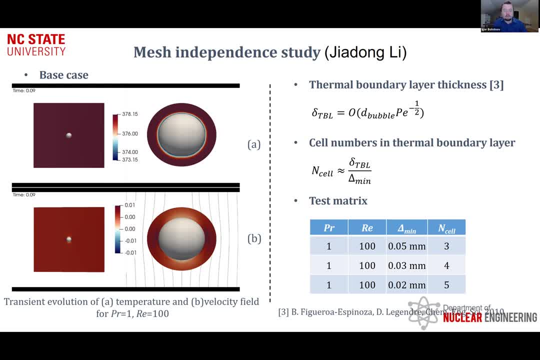 it will get old at some point. but but yeah, we also run on nc state hpc, right. so so those, those single bubble, maybe five bubble type of simulations, it's, it's doable, uh, routinely locally. but but this, this, this large ones, when you're looking at a thousand bubbles, that's when you have to. 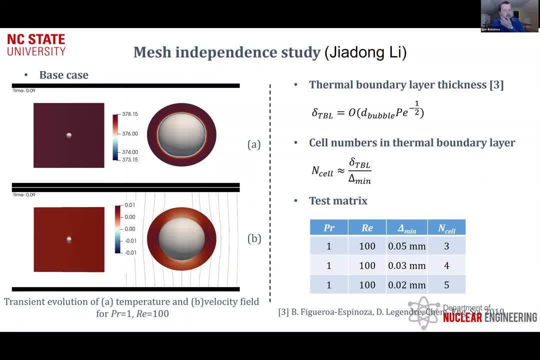 use the large scale. so so whatever like, for example, what, whatever was done at hcdr? again, this single bubble things- they- yeah, they run it actually on on their local machine as well. so a local cluster rubber- yeah, how much of a learning curve is there? i mean, i'm assuming you'll get students who come in. 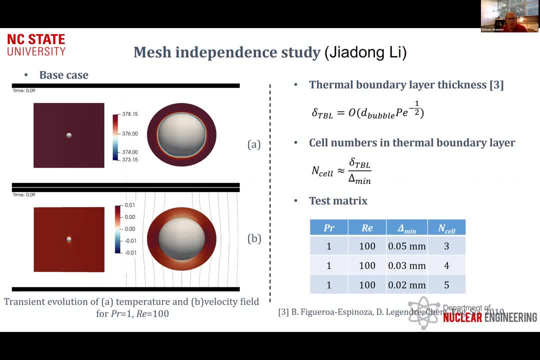 who've done a lot, who've done some simulation work or maybe played around with uh, you know, with, with, with fluid models. but how much of a learning curve is there to you know? upgrade the uh, the simulation, their simulation, knowledge where they can optimize, optimize code for parallel. 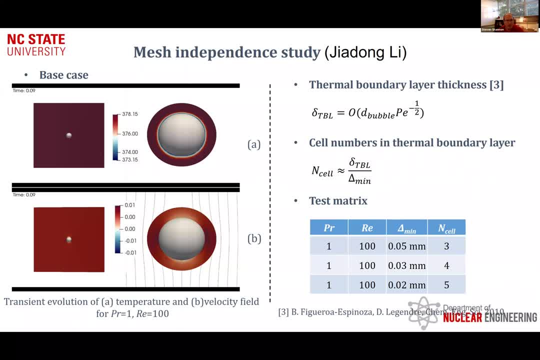 processing. is this something they have to do, or is this, is this, is this already kind of? so it depends on the, on the project. yeah, so typically, um, uh, to use the code, because it's a research code, so it's not exactly your sort of star ccm, right so, which you're supposed to learn in a day. so typically it. 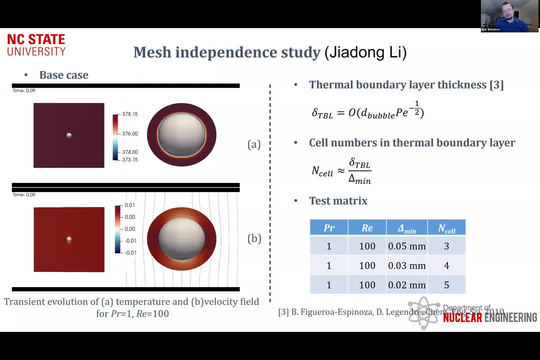 takes a a good student a month or two to sort of get comfortable with all the you know processes, right. but then the next stage is indeed to to not only to uh implement new capabilities right, for example either data analysis or physics-based capabilities like contact angle, but also to rather maintain the um scalability of the code, right. so so, so in 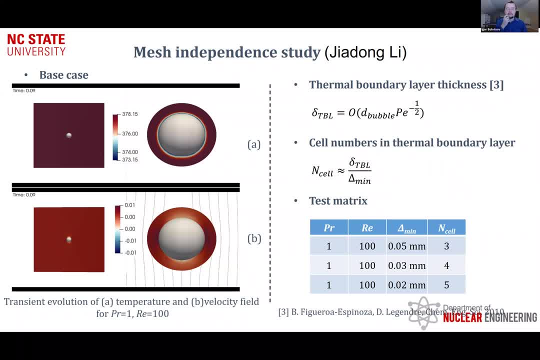 the current version. the code can be scaled quite well, but but you have to make sure that, yes, you learn how to program in such a way, but but you sort of follow the example, but but yeah, that's, uh, that's quite a bit of um, fortran and c and linux and these kind of things. okay, thank you. 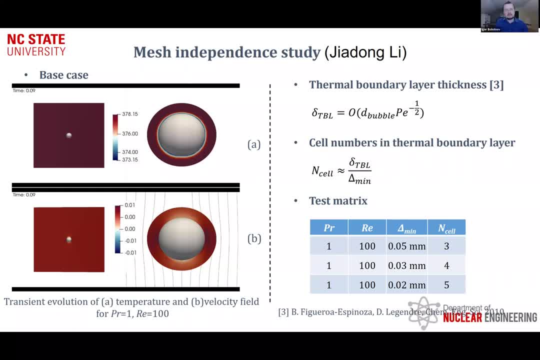 any questions from the audience. i think my win was raising a hand. i saw i don't know what's that. uh, i i had a comment on the just uh nc state hbc is that we are actually actively, you know, debugging uh issues with use on it, but in theory it would form actually a pretty good bridge in between our 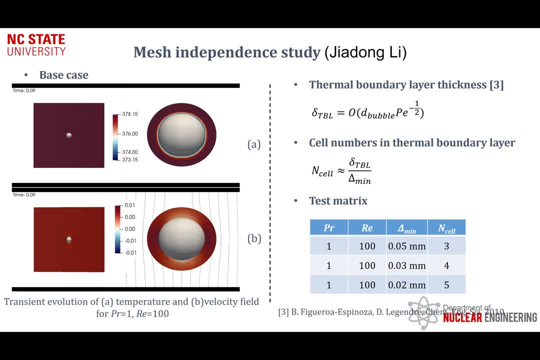 kind of the scale we run locally on our cluster and this the scale we run on, say, argon's machines. um, it would, it would kind of, yeah, it would be a very good intermediary for those too. yeah, yeah, naveen is my, my front man and only insisted hpc he is. uh, yeah, he's bothering them and trying to make. 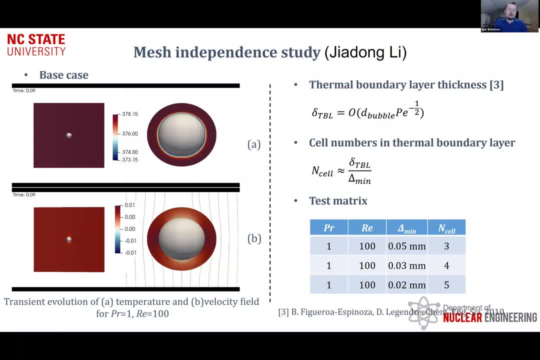 sure to get it to work. yeah, because, and, and then there's the whole, like the, the that's. there's the thing where, like the way the design is, it's like you. you know, we are a project control engineer, but that's my one of the reasons. I mean, we looked into it before, but now again the concern is: 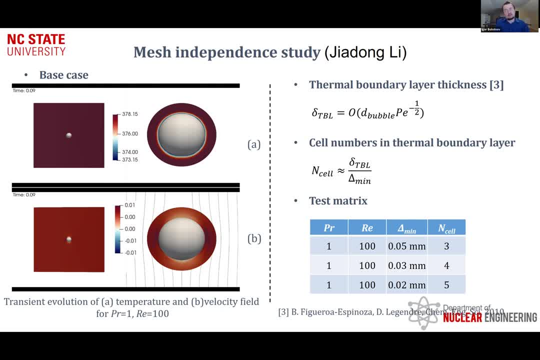 so I got my cluster like eight years ago. so the concern is it may die at some point and then, depending on how much money I can find to, to you know, repair it. yeah, that's gotta have a backup. yeah, that's the challenge, man, computers get old, so yeah, 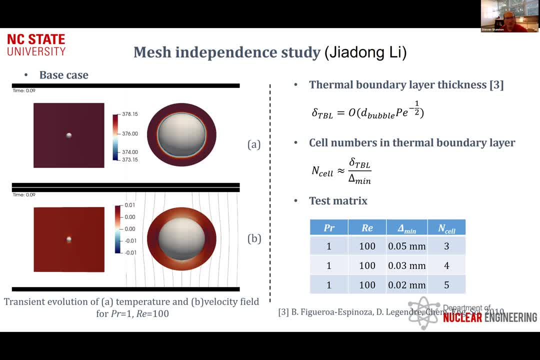 suddenly you guys have the same challenges we have as experimentalists: having to replace very expensive equipment to keep your stuff going. yeah, yeah, no, that's, that's similar, but. but in that sense, no get. but getting those hours is also. that's another challenge actually going into the future. for example, many supercomputers become gpu based and I cannot really write the.